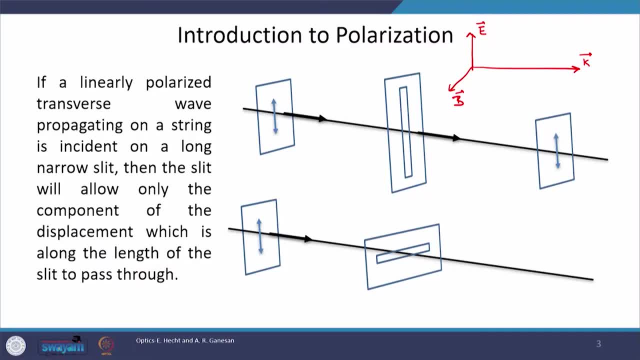 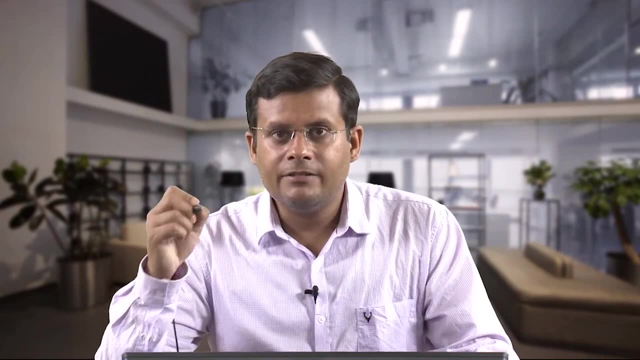 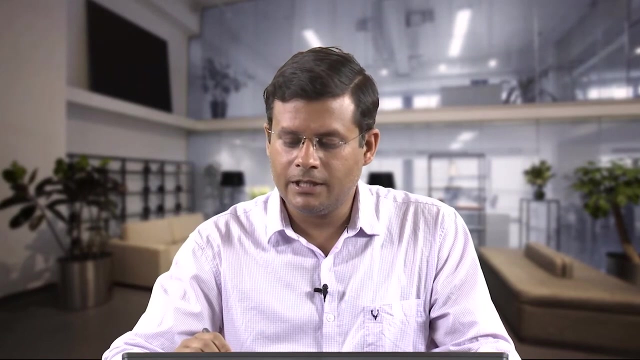 to each other. Alternatively, what we can say is that the E, B and K, the wave vector, they all three must be perpendicular to each other And polarization is always associated with the direction of vibration of E, Because we know the electric. 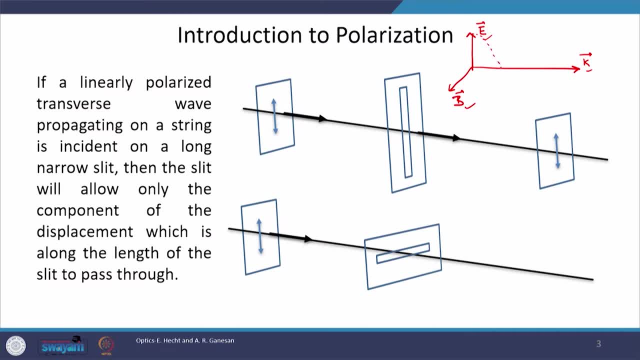 field is a time dependent field in electromagnetic wave. Therefore it will keep varying. Its magnitude is a function of time. It will keep varying, So it is a function of time. It will slowly reduce down and then it will change its orientation and then it will increase. 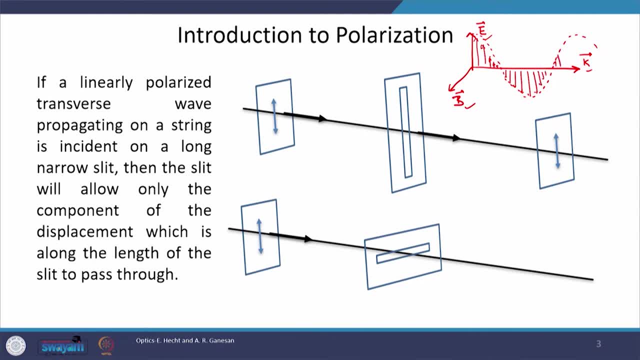 in a reverse direction and then again will go down, And this is how it will oscillate. The electric field vector will oscillate slowly. Similarly, the B field will also oscillate in a plane which will be perpendicular to the E field. B field will oscillate in this. 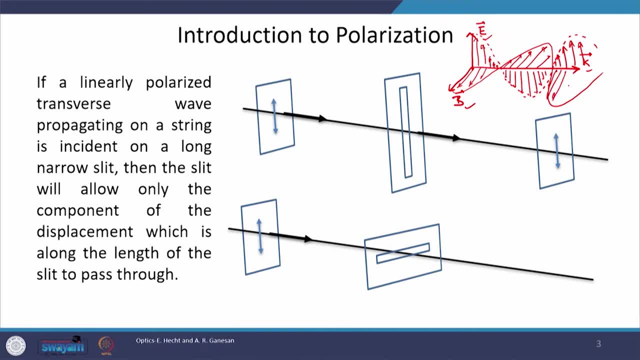 plane, The perpendicular one, And E field is much stronger than the B field And the magnitude of E is related to B through speed of light. in vacuum It means electric field E. the magnitude of E is C times stronger than B. And what is the value of C? C is 3 into 10. 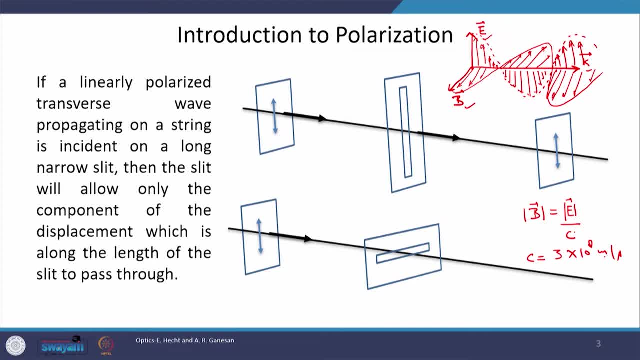 to power 8 meter. So it is a very big number And there is therefore a huge difference between the magnitude of electric field and the magnitude of magnetic field. Therefore, when we shine light on some object, then it is electric field which interacts with the object dominantly, And the interaction 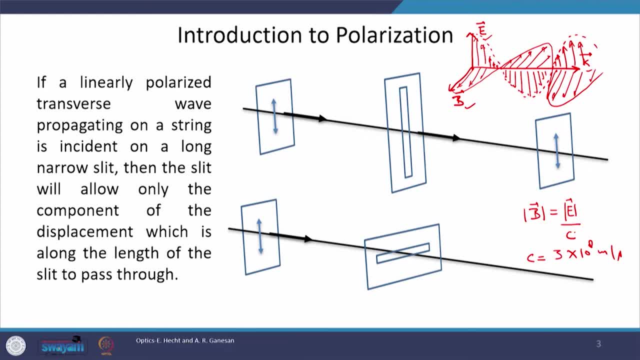 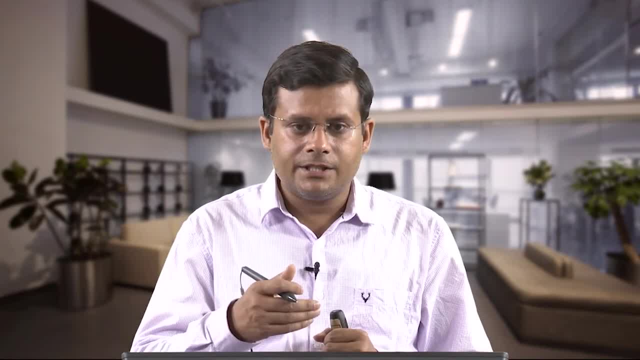 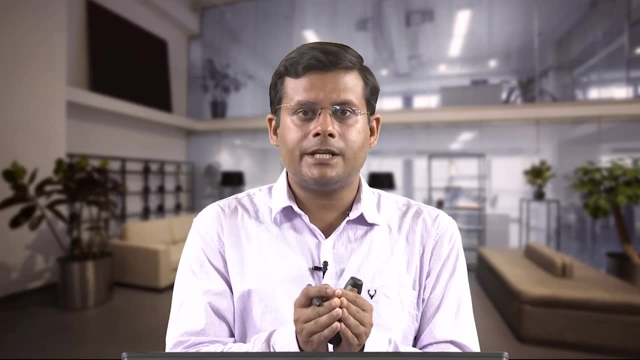 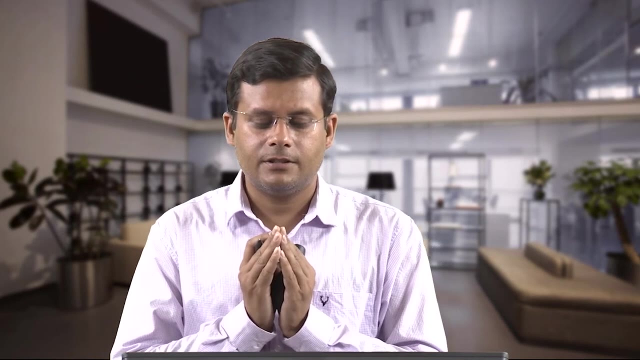 of magnetic field would be much weaker. Now, since the dominant component is electric field, we associate polarization with the E field. Therefore, whenever we say polarization, it means a quantity which is directed along E, the electric field. Now you see that in. 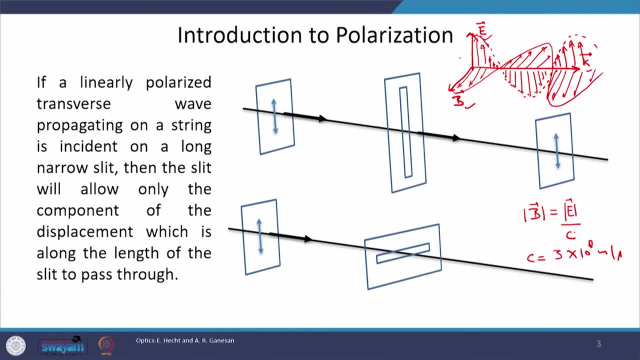 this figure, the electric field oscillations. let us pick different color. The electric field oscillation traces a curve, and which is in a plane, and this plane is plane of the paper, while the magnetic field oscillation traces a curve, which is again in a plane, but this plane is. 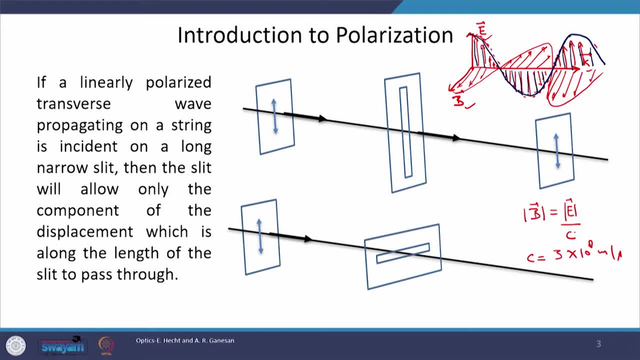 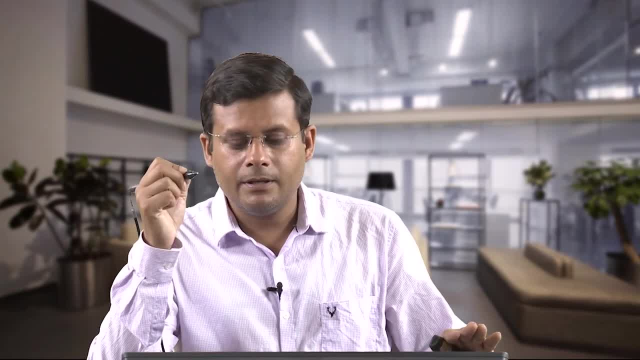 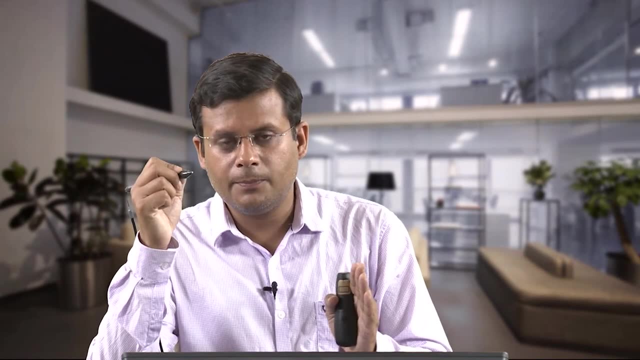 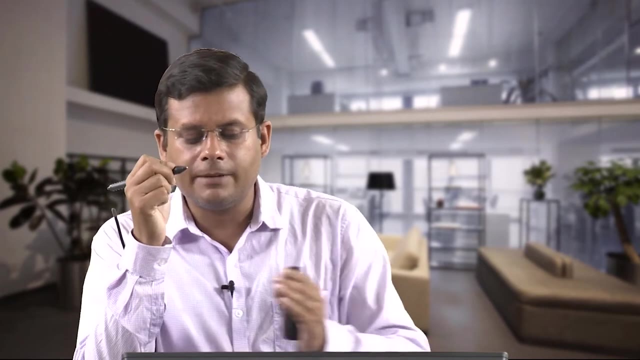 perpendicular to the plane of the paper. Now, the plane created by electric field oscillation is in the plane of the paper and if we see, we say that polarization is along E, then with propagation this polarization is creating a plane And therefore this type, this particular type of polarization, is called plane polarization. 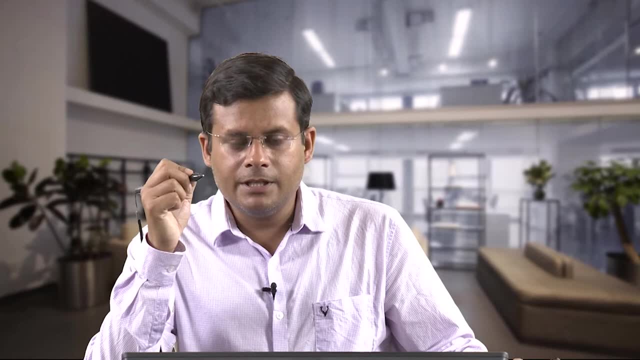 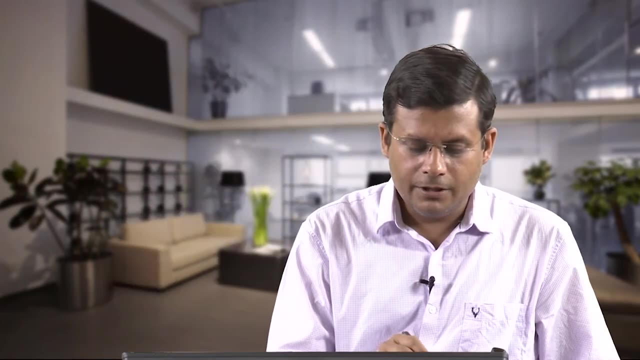 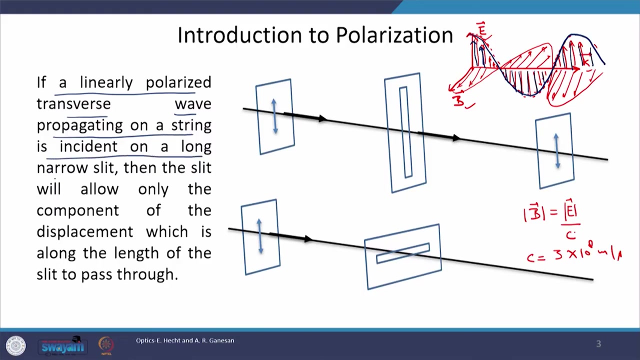 or the wave is said to be linear, linearly polarized wave or plane polarized wave. Now, if a linearly polarized transverse wave propagating on a string is incident on a long, narrow slit, as is shown here, this is a opening of certain width and a wave who is polarized linearly. 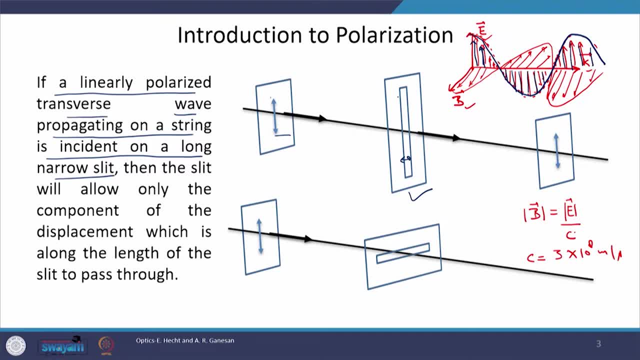 and its oscillation, The direction of polarization. Polarization is along the length of the opening, along the length of the slit, then whole of this oscillation will pass through, And if there is some rotation of the oscillation or of this narrow slit, then it will stop the component of the wave. It means, or we can. 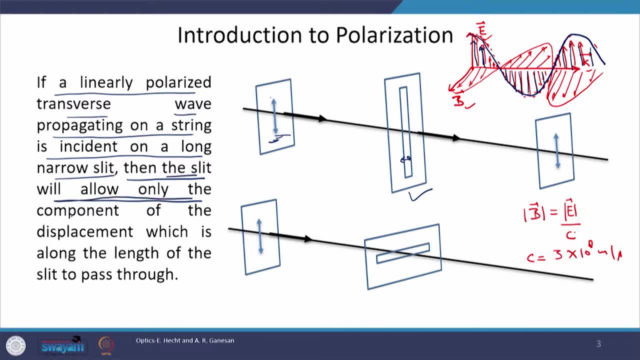 say that the slit will allow only the component of the displacement Which is along the length of the slit to pass through. And if the slit is allow, allowing this particular oscillation, then we can say that at that instant the electric field is oscillating along the length of the slit And such a slit will convert a unpolarized 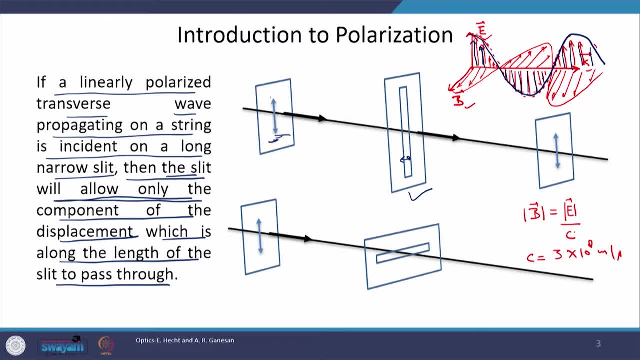 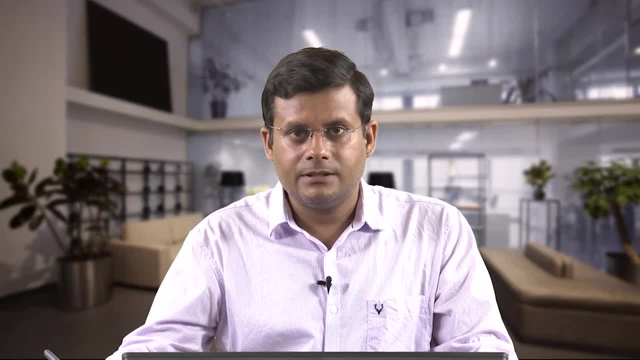 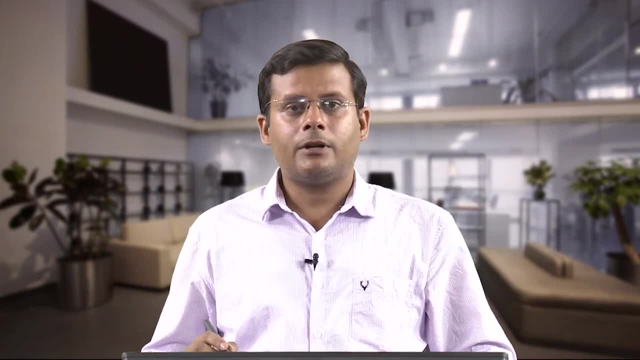 wave From a unpolarized light to a polarized light, or, more accurately, to a linearly polarized light or to a plane polarized light. Now, what is the difference between unpolarized light and the linearly polarized light? then, Now we know that electromagnetic wave is a transverse. 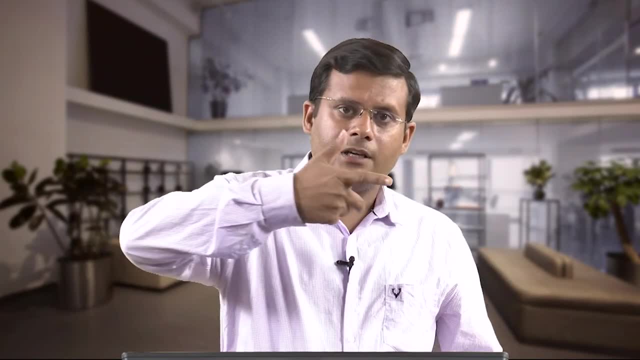 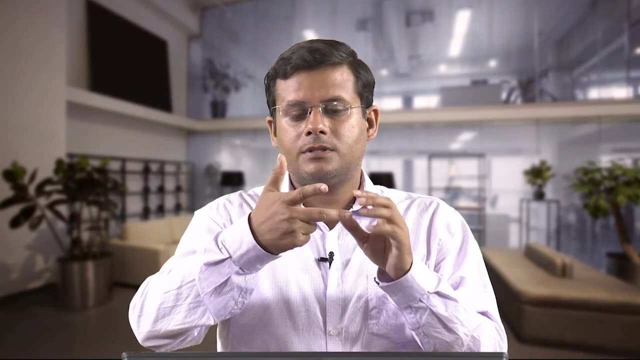 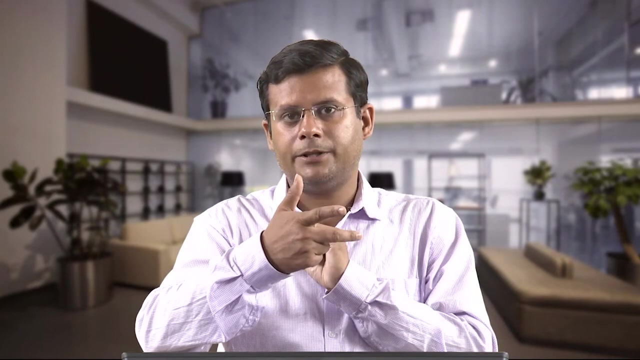 wave and it has a certain direction of propagation. and perpendicular to the direction of propagation, we have electric and magnetic field orientation. Now, since E and electric field and magnetic field are functions of time, they will keep changing their amplitudes, But they may take any orientation while propagating along the 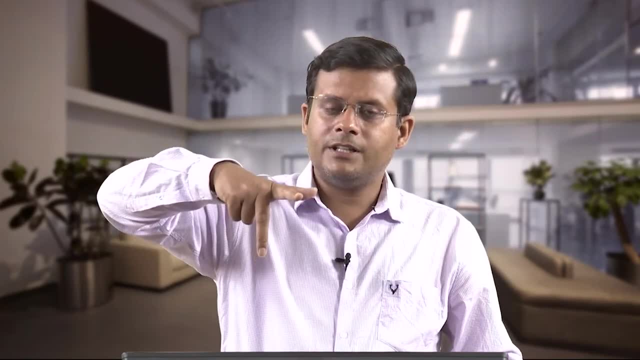 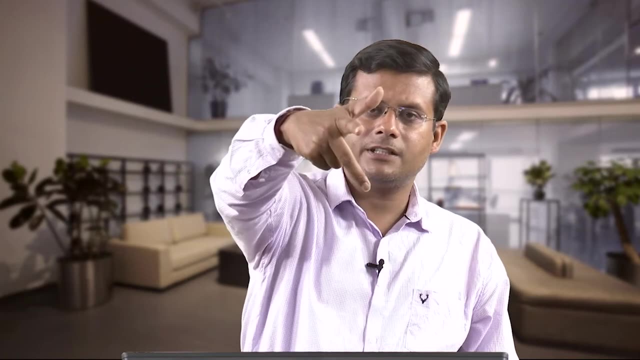 medium They may. at one instant of time they would be oriented like this, while on the other instant they may take this orientation, In the next instant they may take this orientation. The orientation of electric and magnetic field is completely random. Now, if you take this, 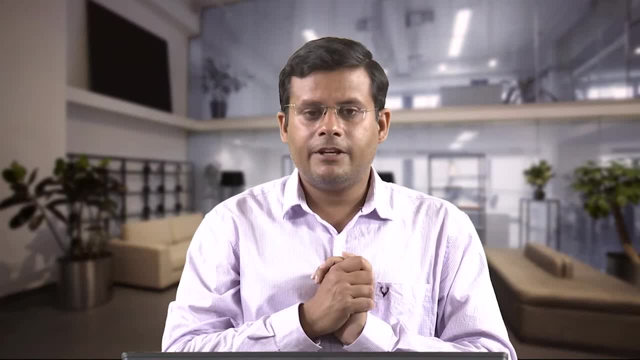 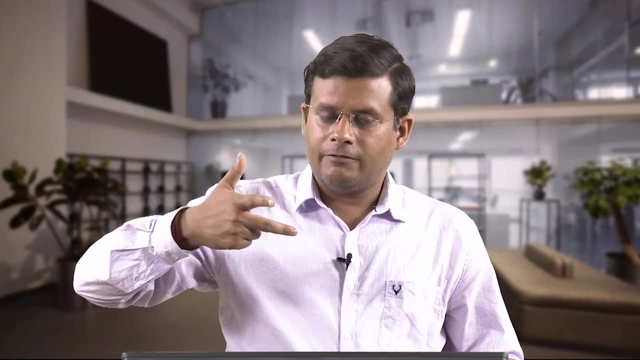 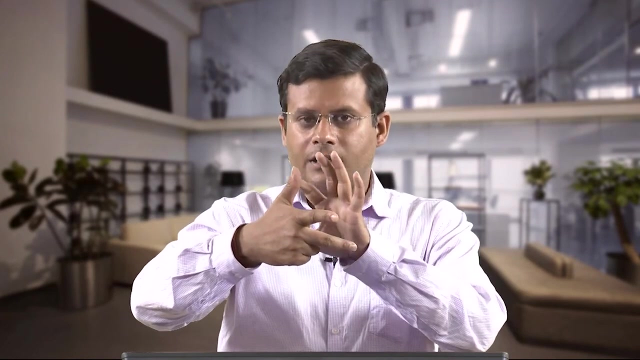 orientation of electric and magnetic field. and magnetic field, it is completely random And if this is the case, the wave is said to be unpolarized, While a wave which is propagating, which propagates like this, are a waves in which the electric field vector oscillation. 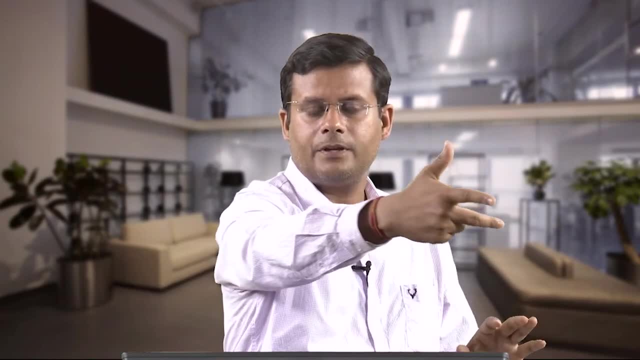 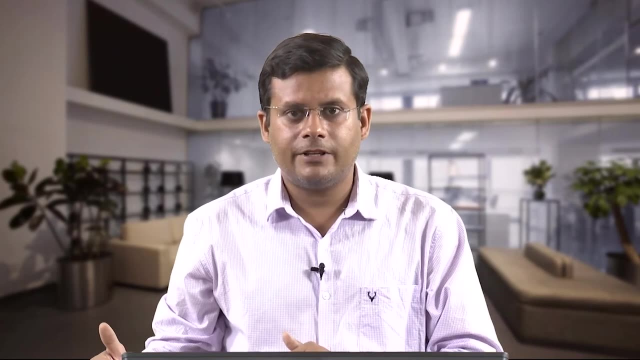 of electric field vector traces a plane with propagation. Such a wave is called linearly polarized light or linearly polarized wave. Lecture 10, Lecture 11, Lecture 12. Lecture 13, Lecture 14, Lecture 15, Lecture 17, Lecture 18. 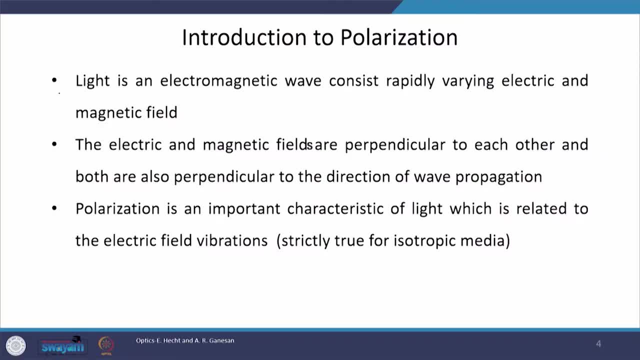 Lecture 19. Now let us go deeper into this concept. The first thing which we should understand is that light is an electromagnetic wave And it consist of rapidly varying electric and magnetic field. since electric and magnetic fields are time dependent, therefore they vary very rapidly. The electric field and magnetic field are perpendicular to each other. this 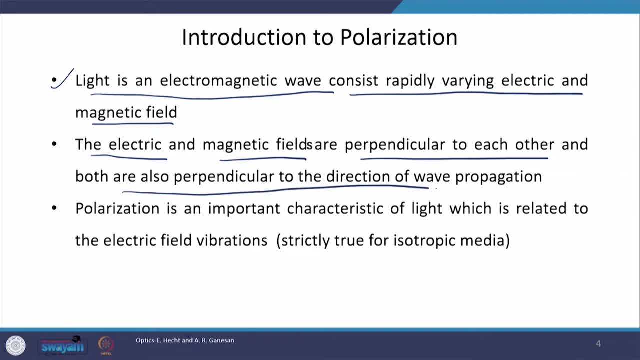 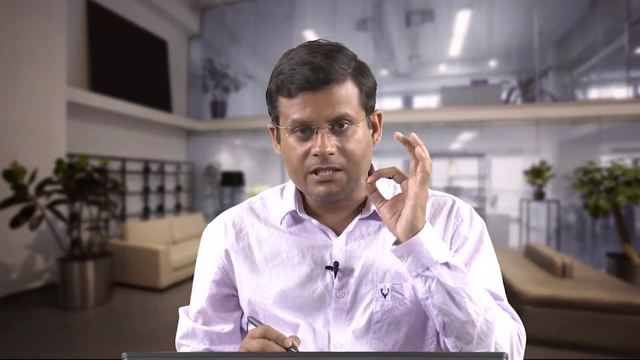 we have understood, and they both are unpolarized, also perpendicular to the direction of propagation of wave, And polarization is an important characteristic of light which is related to the electric field vibration. It is always along the E field orientation, But this statement is strictly true for isotropic media, As discussed. 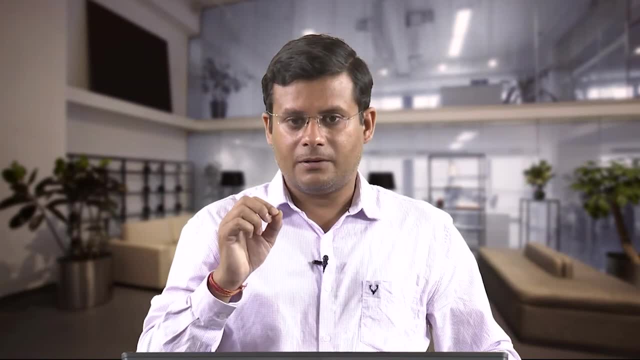 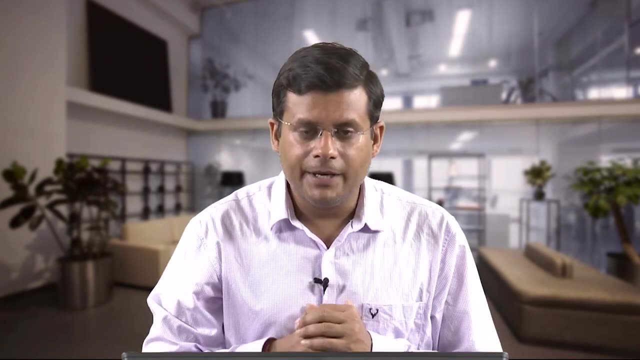 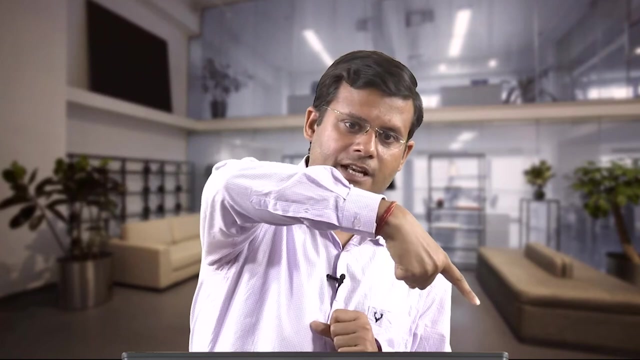 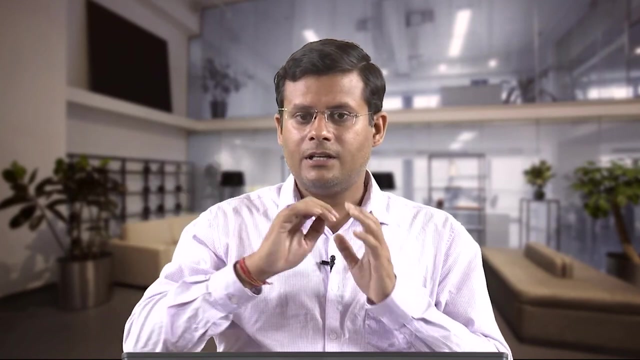 earlier. isotropic materials are materials in which the properties of the medium are not direction dependent. The isotropic medium will have same property in this direction as well as in this direction as well as in this direction. In all the directions, the isotropic material will exhibit the same properties. 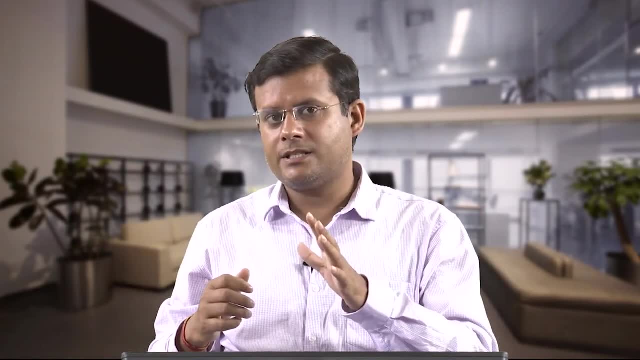 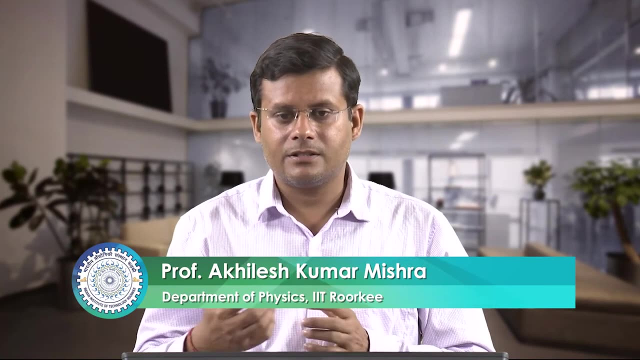 While in anisotropic medium the properties of the material will not be direction dependent, In anisotropic material the properties, the optical properties of the material become direction dependent And these materials are called anisotropic. Now for isotropic material. 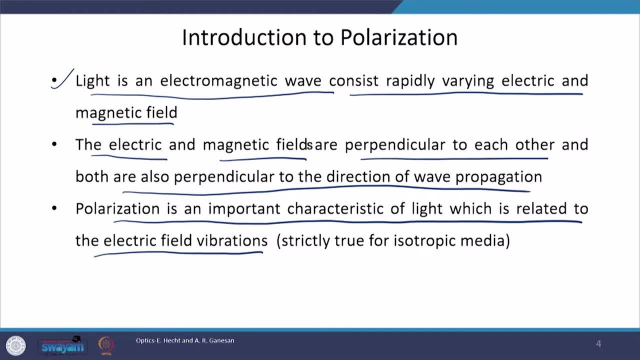 this definition holds very good. We will talk about anisotropic material in our later classes, But for now on, it is correct to associate polarization with the direction of E field. Why? Because E field is dominant as compared to the other field, which is our magnetic field. 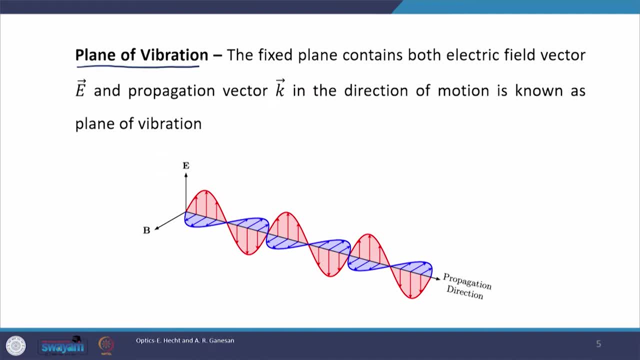 Now, before moving ahead, we must understand what is plane of vibration. The plane of vibration is defined as a fixed plane which consists both electric field vector E and propagation vector K, And from this figure, what you can see is that the electric field vector E is. 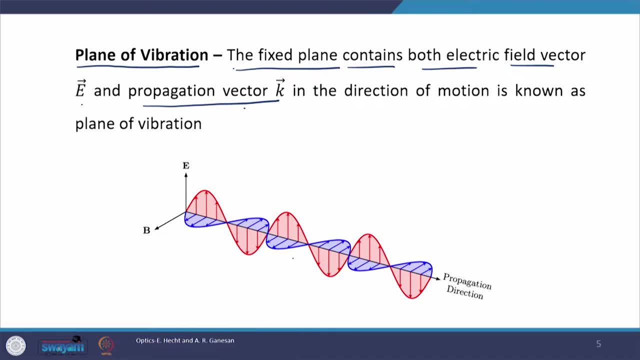 C is that the red curve, the red curves, shows the evolution of tip of electric vector, while the blue curve traces the tip of B field, the magnetic field. Now, this vertical direction is the direction of E and this is the direction of propagation, The direction of propagation. 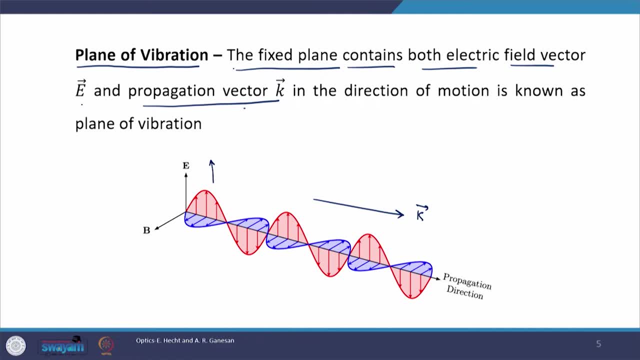 is represented by propagation vector K And K is this and a unit vector, say. A Unit vector is a vector quantity which indicates the direction and mod of K. is K which we already defined, which is equal to 2 pi by lambda, And the vector nature is coming from this A cap which 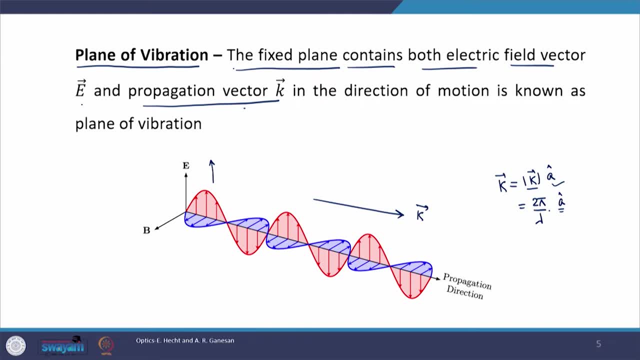 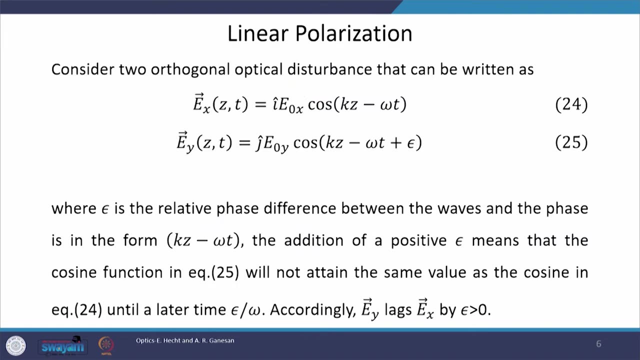 is unit vector which is in the direction of propagation: E. Now, using E and K, we can trace a plane, and this plane is called plane of vibration. Now, once the plane of vibration is understood, let us move further in understanding the concept of polarization, or, in particular, linear polarization. mathematically. Now consider two orthogonal 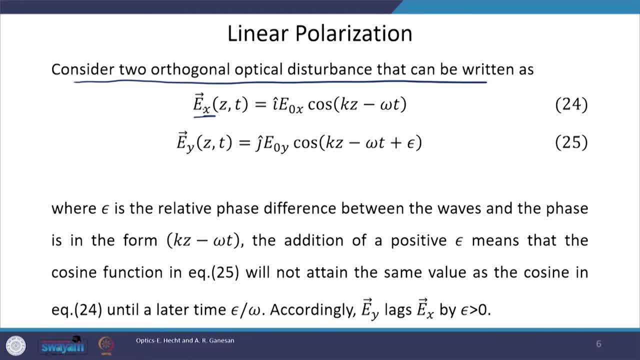 optical disturbances. • E, E, E, E, E, E, E. Now first is E and second is E. E and represents the direction of vibration. It means that E represents a field which is oscillating along x axis and E represents a field which is oscillating along y axis. and 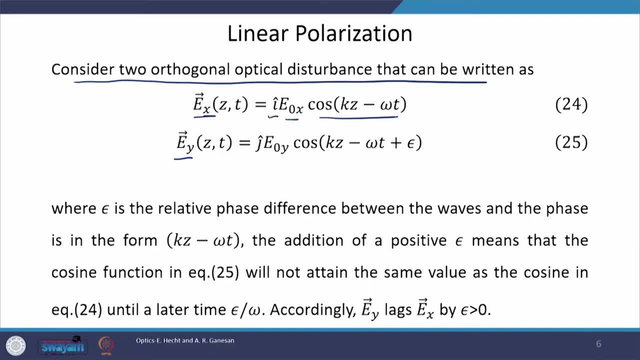 E is equal to I cap E naught x. cos kz minus omega t? kz minus omega t is phase light minus kz minus omega t, m, k and d, m, k and d for kz. So kz minus omega t is the average wavelength. 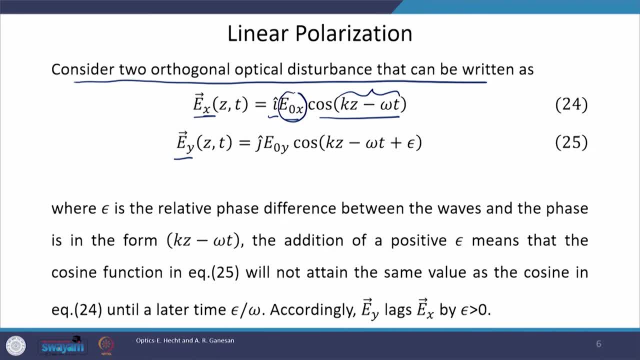 group, So they not shift going towards this D group. Now, now the first oppositeNathan A, f by e naught. x is amplitude and i cap is nothing but unit vector along x axis. Similarly, the expression for e, y is equal to j cap, e naught, y, cos, k, z minus omega, t plus epsilon. here. 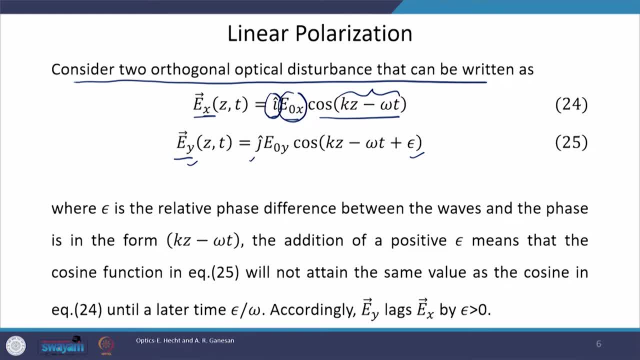 again, j cap is nothing but unit vector along y axis. e naught y is the amplitude, and k z minus omega t plus epsilon is phase. But here epsilon is the relative phase difference between the two waves and the usual phase is in the form of k z minus omega t. Now the addition of a positive phase, which is epsilon. 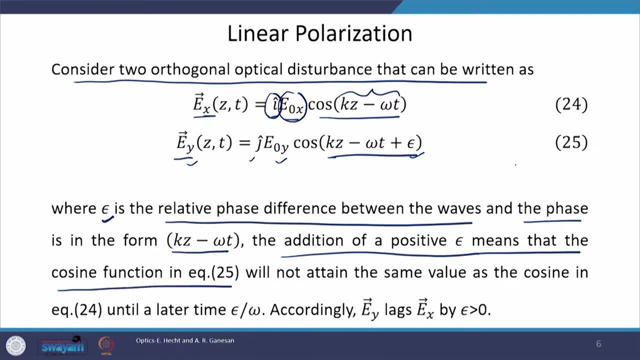 means that the cosine function in equation number 25 will not attain the same value as the cosine in equation number 24.. Let us understand it in a different way. We can write equation number 25 as j, cap, e naught y cosine of k- z. Let us take omega out of the bracket and then we will have t minus. 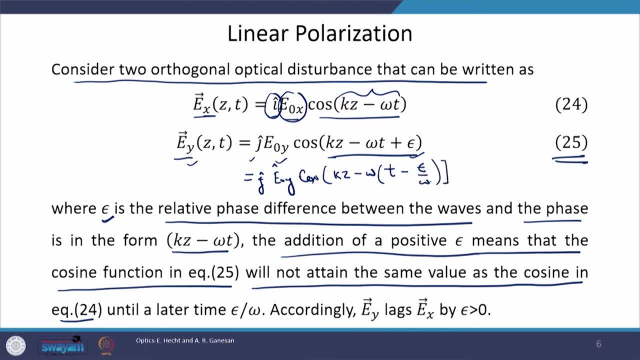 epsilon by omega. This is the modified expression. Now, if you compare equation number 24 with this modified expression, then what you see is that in equation 24 the phase part is k z minus omega t, while in this modified equation 25 the phase part is k z minus omega in bracket- t minus epsilon. 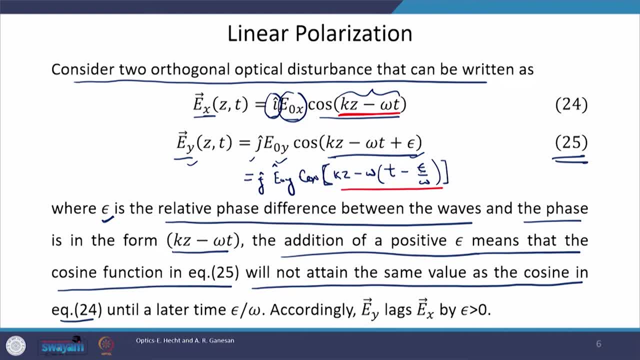 by omega. This epsilon by omega factor is being subtracted from time. It means in equation number 25, the overall phase is running slower, It is a behind. And this is what is what exactly is being said in the line here: The addition of a positive 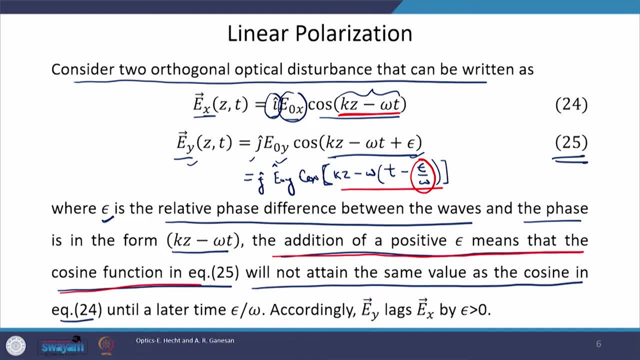 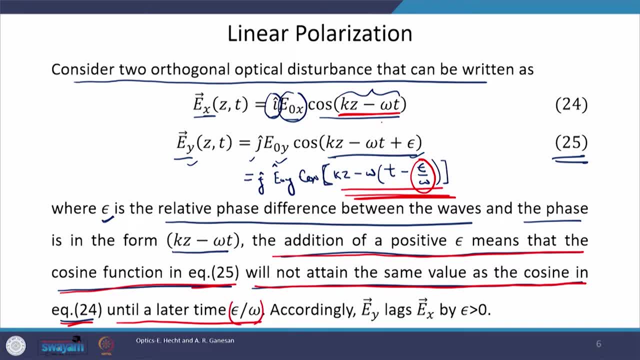 us see回 aاد losu. is this one count of minus 힘 epsilon by omega? Equation number 24 has this phase. It evolves in time And the same phase would be achieved by equation number 25 only after an additional time. and this additional 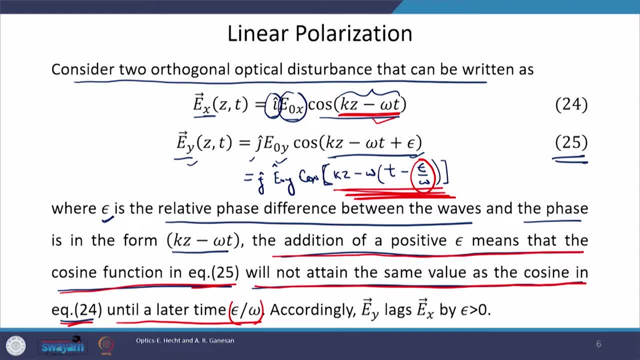 time is epsilon by omega, which clearly says that equation number 25 is lagging behind this one count behind equation number 24, or in other words, E? y is lagging behind E x. provided epsilon is larger than 0, E y lags E x by epsilon. Now, if epsilon is negative quantity, then 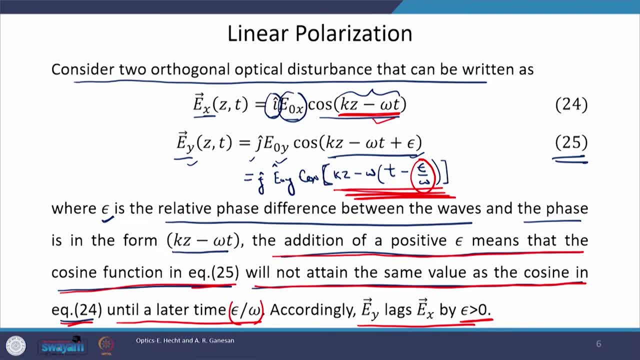 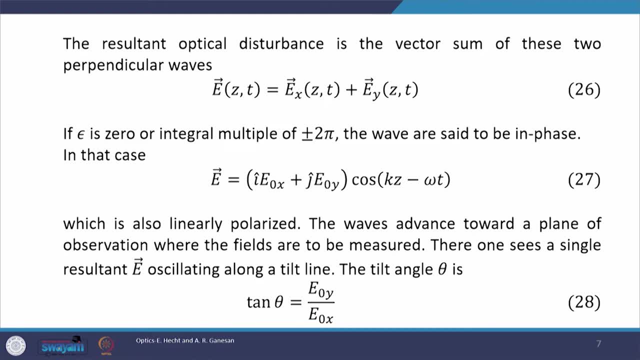 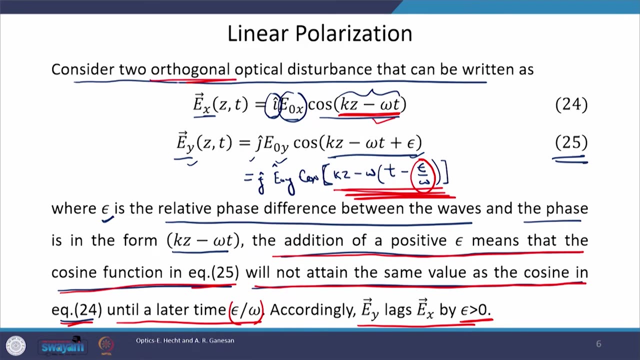 E x will lag E y. yeah, Now let us calculate the resultant. how to calculate the resultant? we will again resolve to superposition principle. we will add these two waves. Now you, as in the previous slide, we assume that these waves are orthogonal and they. these are the fields. 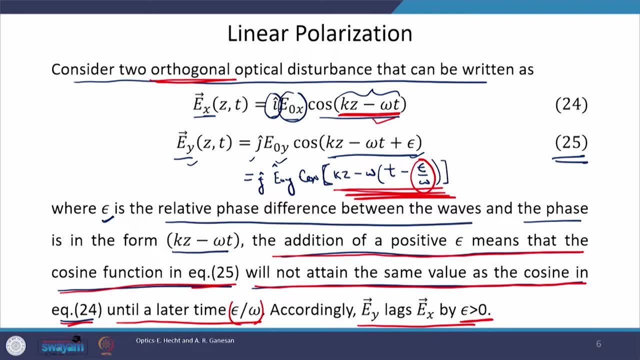 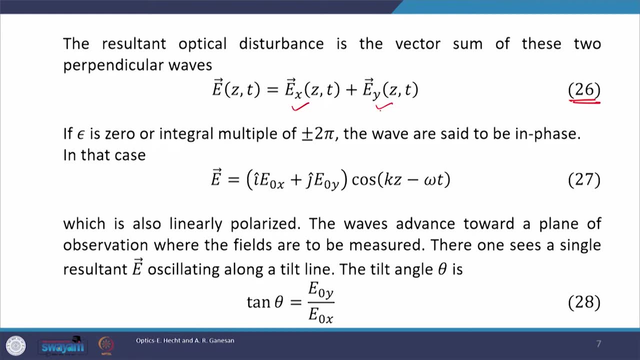 which are vector quantity, And therefore we will have to take into account this vector nature and this addition would be vector addition. Now, here, in equation number 26, we are adding E x and E y vectorially, because these are two perpendicular components here E x is perpendicular to E y. Now if 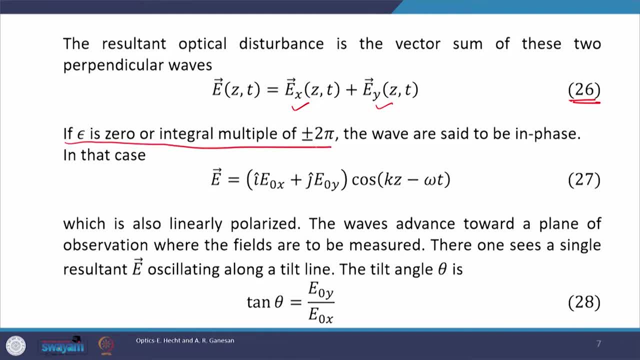 epsilon is 0 or integral multiple of 2 pi, The waves are set to the in phase. we know it. yeah, we understood it in our last lecture. okay, Now, in the case when epsilon is either 0, epsilon is our initial phase. if epsilon 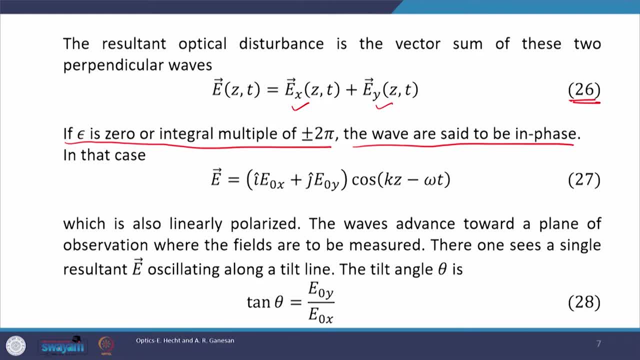 is either 0 or multiple of plus minus 2 pi, integral multiple of plus minus 2 pi, then the resultant will have this expression, which is given by equation number 27.. And the resultant and e is equal to i cap e, not x, plus j cap e, not y, and the phase part is cosine kz, minus. 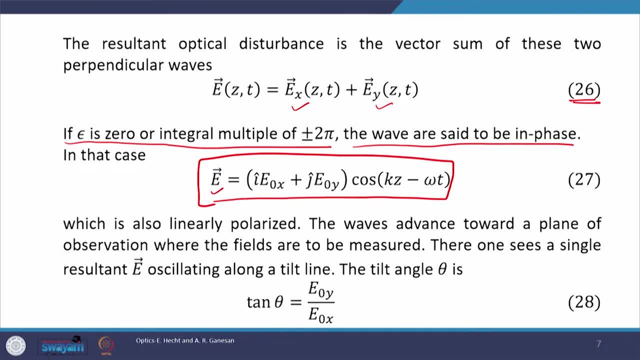 omega t. okay, Now, what is the state of polarization of this resultant wave? How to know about this? Now, you see that it is a vector addition. We are adding e, x and e y. Then let us plot it here. If you plot it, let us put e x on x axis and e y on y axis. okay, Now the magnitude. 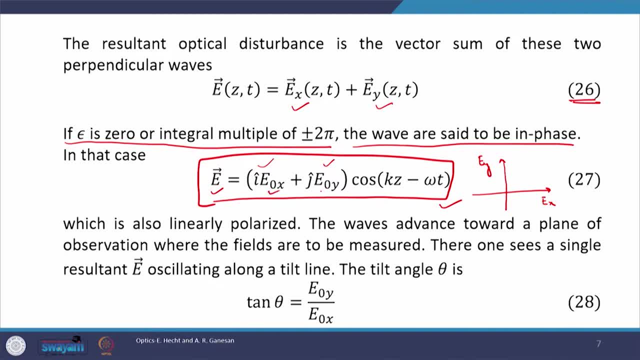 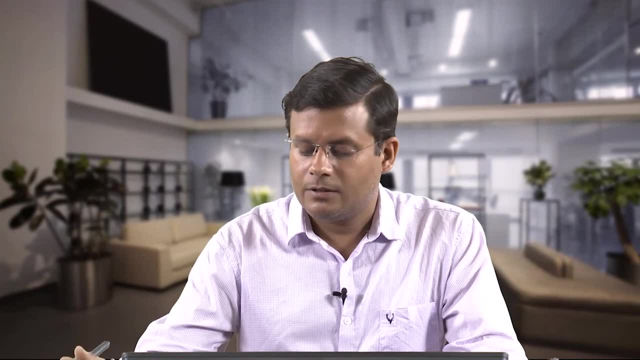 here is e not x along x axis and e not y along y axis. okay, There would be some magnitude here in x direction and some magnitude here in the y direction, and the resultant would definitely be pointing here And it would… It would be in the… The resultant will oscillate in first and third quadrant. yeah, This would. 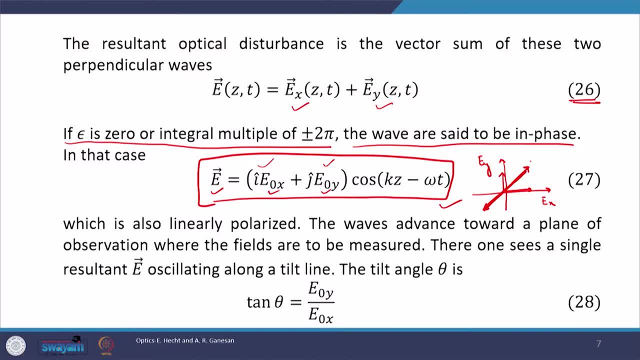 be the oscillation direction of the resultant. That would again be a linearly polarized wave, is not it? Because the resultant oscillation is again linear, It is confined to a certain plane and with propagation this linear oscillation will generate a plane. Therefore this wave, 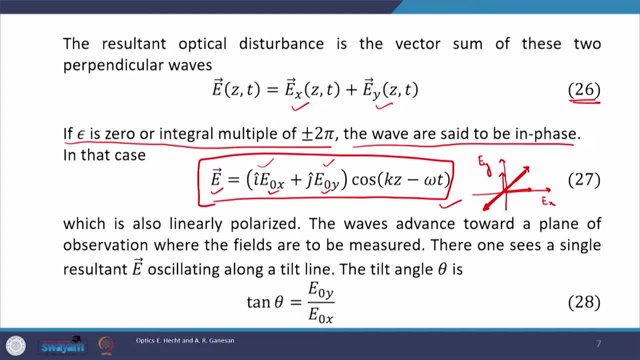 is plane polarized or linearly polarized? okay, The wave advance…. The waves advance towards a plane of observation where fields are to be measured. yeah, There one sees a single resultant e oscillating along a tilt line. okay, You see that the 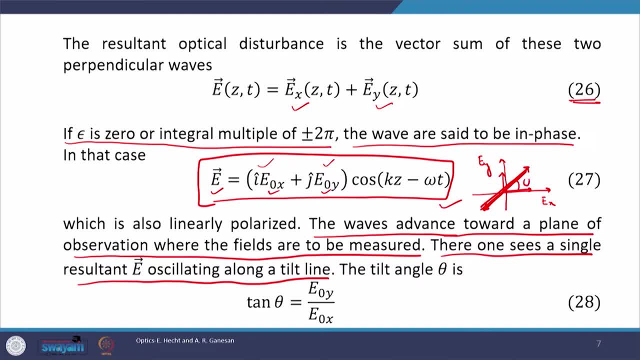 resultant is oscillating here, but it is tilted by an angle: theta. How to know theta? Very easy. yeah, This is how we can calculate theta. How it is done, It is a…. We have two part: e naught, x, cos kz minus omega t and e naught. 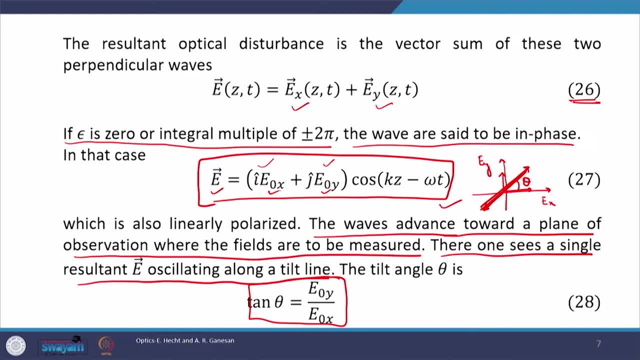 y cos kz minus omega t. y by x will give us the angle. yeah, If you want to calculate theta, how to calculate? Take y component and divide it with x component. The y by x value will give you tan theta. This is what is done here. okay, e naught. x cos kz minus. omega t. This is what is done here. okay e naught x cos kz minus omega t. This is what is done here. okay e naught x cos kz minus omega t. This is what is done here. okay e naught. 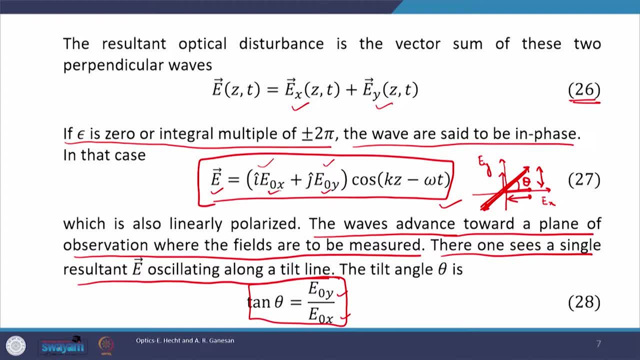 E naught cos k z minus omega t is kept in numerator and E naught x cos k z minus omega t is kept in the denominator and cos cos will go away, and then tan theta would be equal to E naught y upon E naught x, which are nothing but amplitudes of E y and E x respectively. 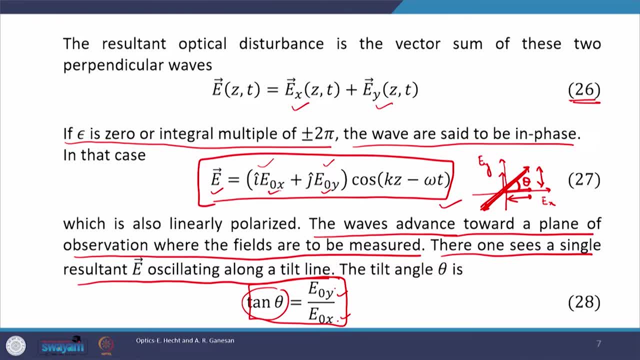 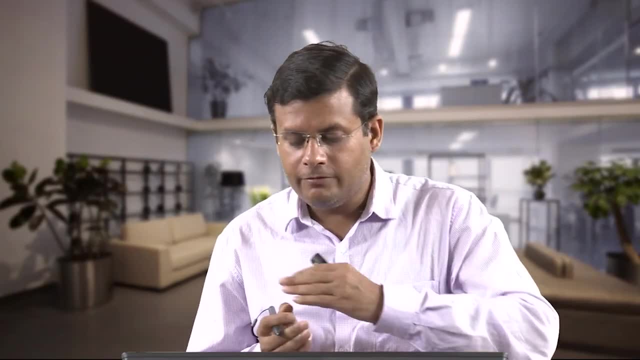 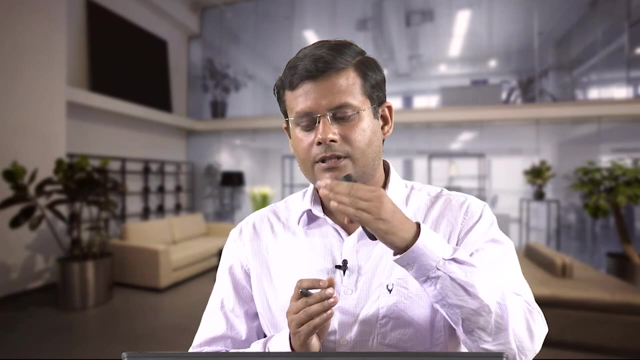 From here we can get the orientation of the resultant E, y. Now this angle, as you can see from equation number 28, it depends upon the amplitudes. Now, depending upon the relative amplitude of the two wave, the resultant will change its tilt. 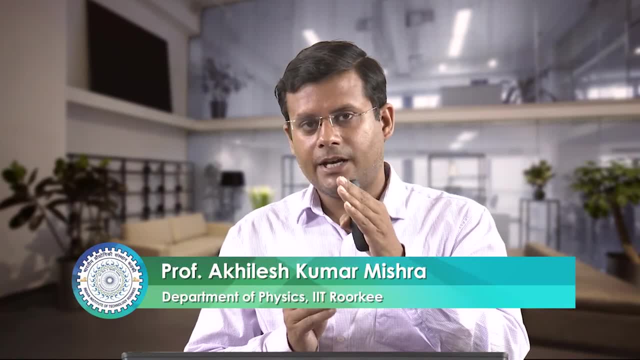 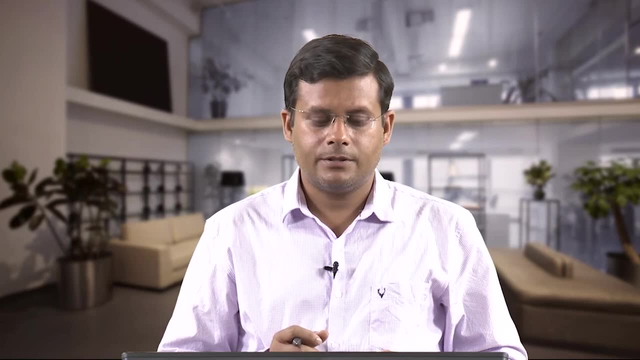 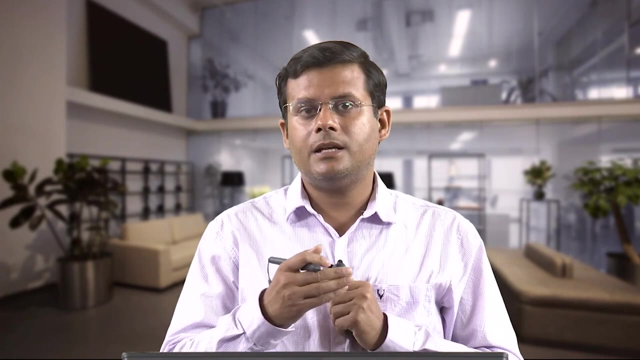 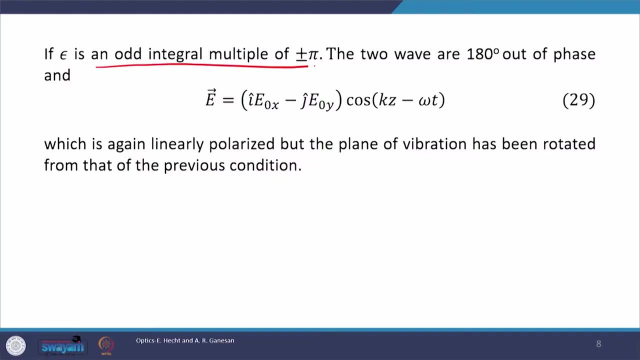 The theta value will vary, and this variation would be directly proportional to the relative amplitude of the two waves. Now let us consider another case. till now we were considering that epsilon is either 0 or integral multiple of 2 pi. What if epsilon is an or integral multiple of plus minus pi? 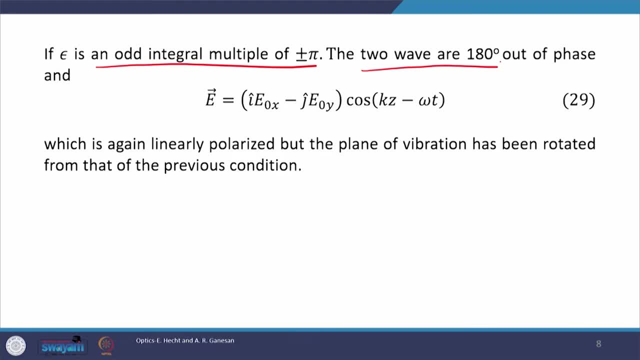 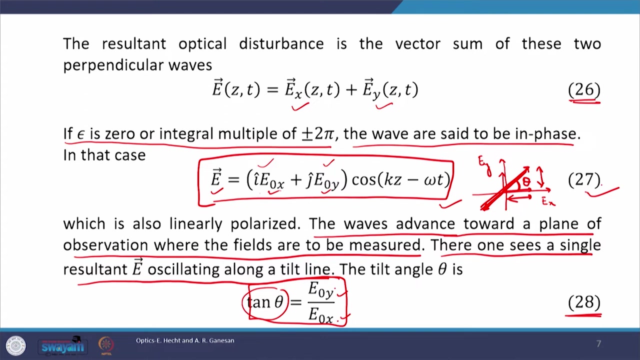 Under this case the two waves will be out of phase by 180 degree by pi radian and the resultant now will be expressed. Now will be expressed differently and this is expressed here by equation number 29.. And the difference between the previous resultant disturbance, which is given by equation number 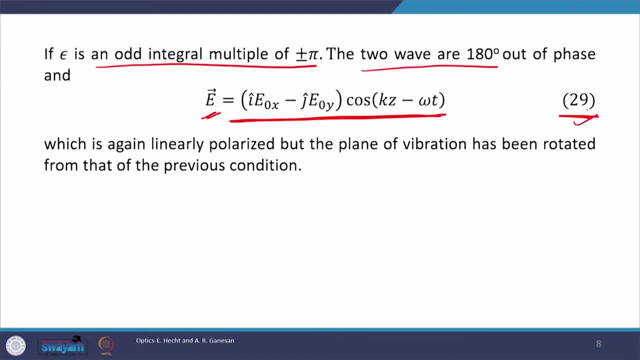 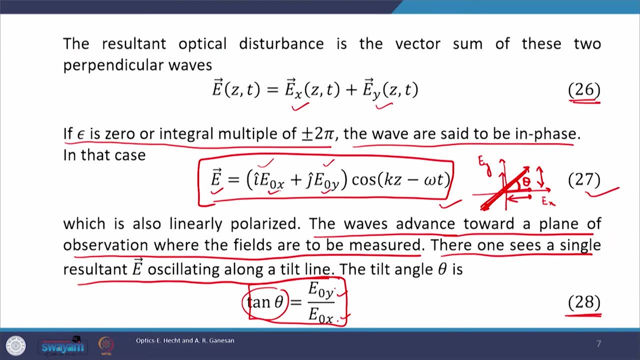 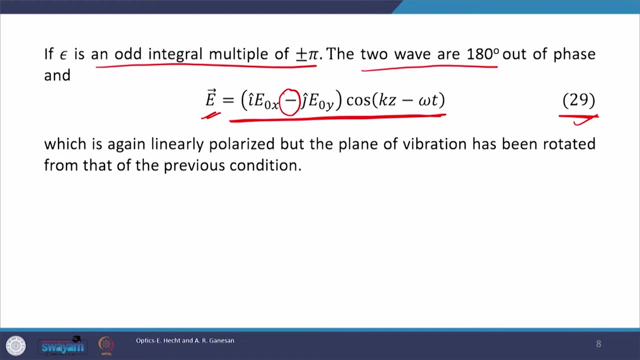 27, and this new resultant is that there is minus sign instead of plus sign Here in equation number 27,. you see that there is a plus sign, while in equation number 29, you see there is a minus sign. How would it? 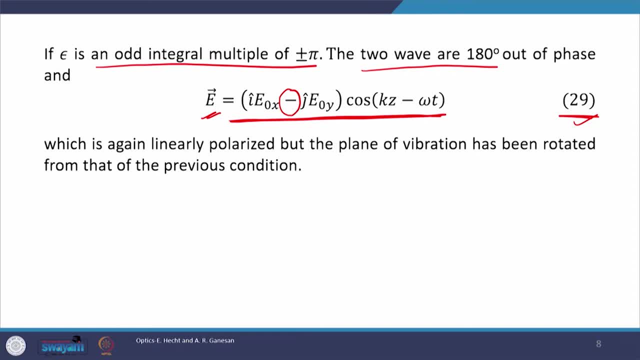 Introduce a difference. now let us again plot Ax and Ey, Ax here and Y component here. What will happen here? The plane of vibration now the resultant here. you see, it will now be in this, along this line. This would be your resultant. 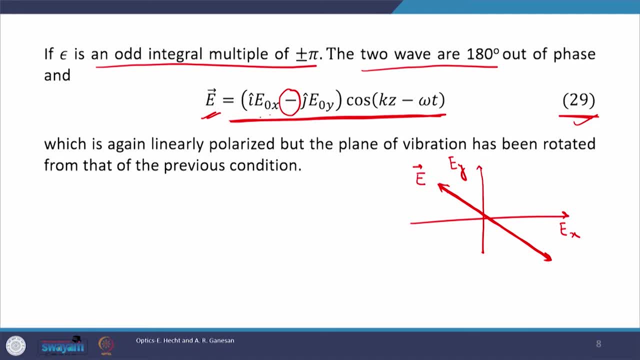 Why? Because X, the Y is minus here, Y component is in opposite direction. X is pointing here at particular instant, Y is here. The resultant therefore would again be, although linearly polarized, but plane of vibration has now been rotated from that of the previous condition. 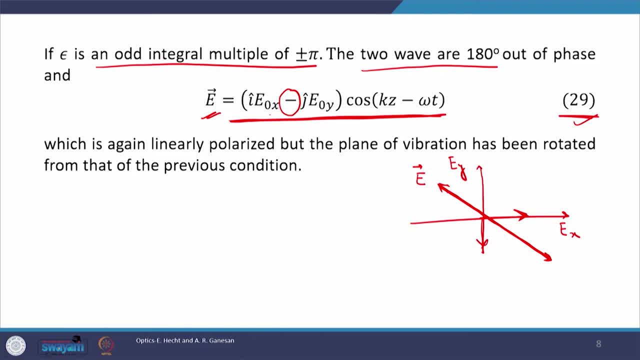 Resultant. Okay, So the resultant is again a linearly polarized light, but there is a rotation of plane of vibration. Okay, Now you see that whenever we represent a plane polarized wave, the resultant always looks like a double headed arrow. 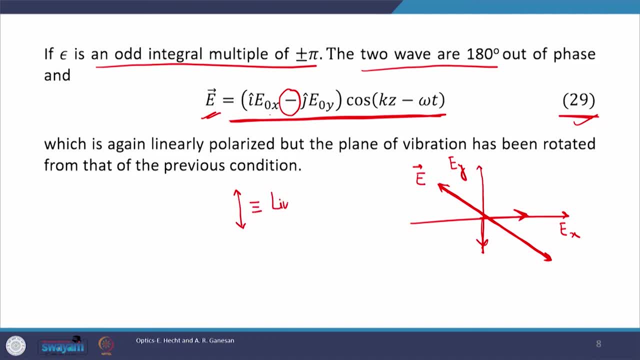 What does this represent? A linearly polarized wave or a plane polarized wave? Okay, So this is the plane of vibration. This is the plane of vibration. This is the plane of vibration. Okay, Now, if this is the representation of a linearly polarized wave, what will be the representation? 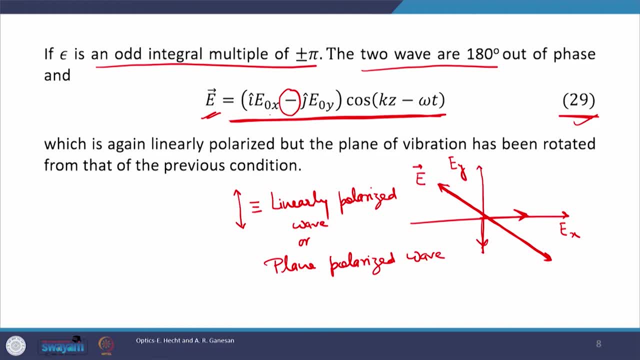 of a unpolarized wave. Now, since in an unpolarized wave the electric field vibration can take into account the vibration, vibration can take any orientation. therefore, usually the convention to represent an unpolarized light is this: Okay, This is used for unpolarized light. 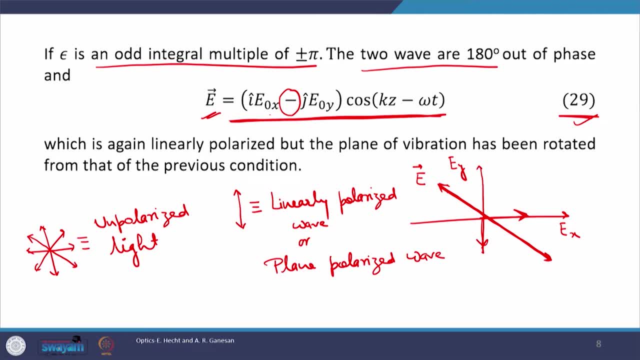 Okay, Single double headed arrow stands for a linearly polarized light. Okay, Single double headed arrow stands for a linearly polarized light. Okay, Single double headed arrow which forms star like a structure. it is used for unpolarized light. 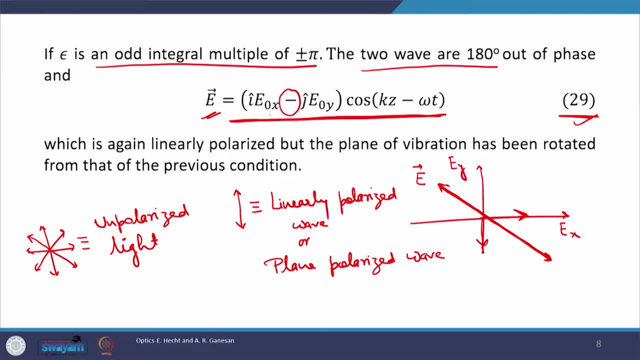 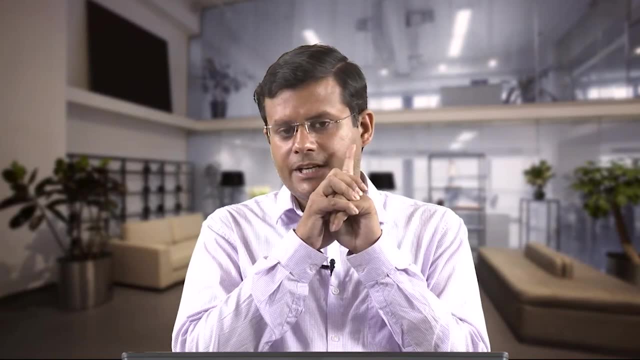 Now, after this analysis, what we can see is the following, In an unpolarized light: if you know the orientation of electric field at a particular instant of time- suppose t is equal to t naught- then you cannot predict or you cannot forecast. 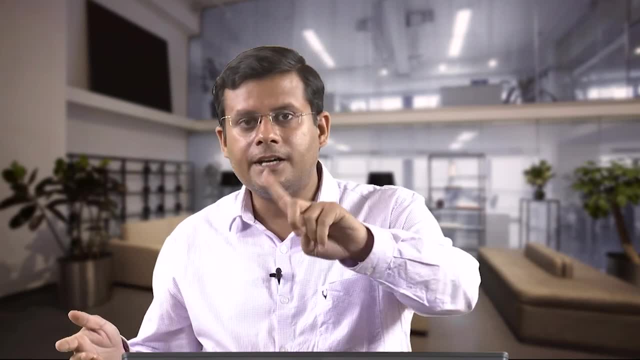 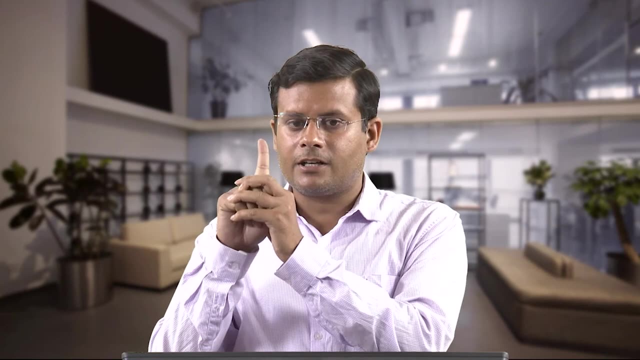 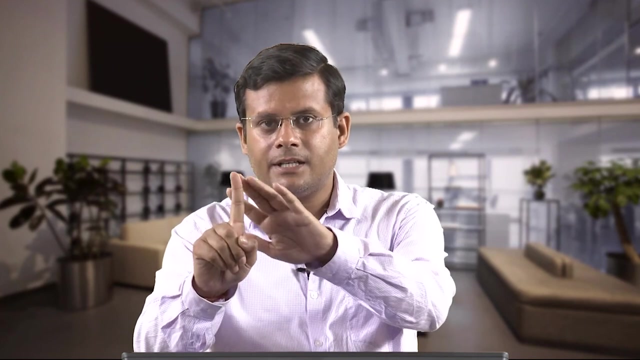 the orientation of electric field at a later time, While in a linearly polarized light, if you know the orientation of electric field at some time- t is equal to t naught- then at a later time you can predict its orientation. 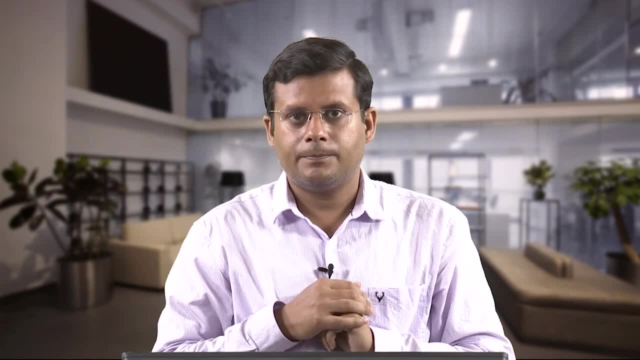 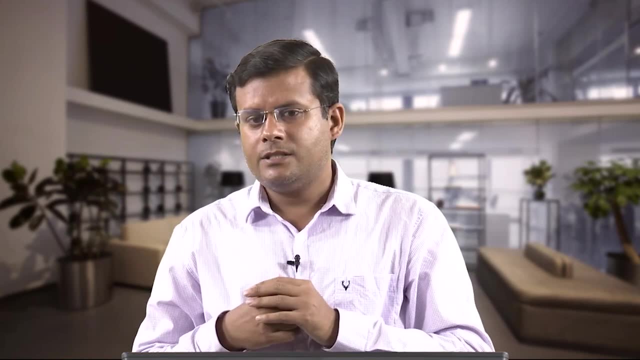 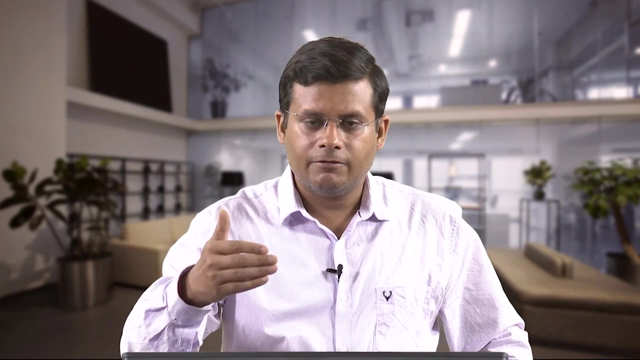 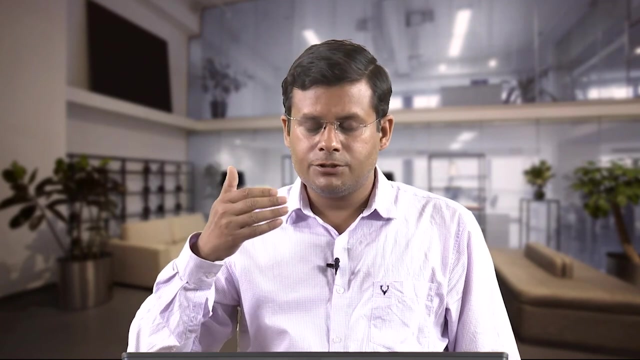 You know that it will always be in the same orientation, Okay. It means that we can say that once a wave is polarized, Okay. Once it is polarized, the predictability comes in our hand If you can predict the orientation of the electric field. once you know the orientation, 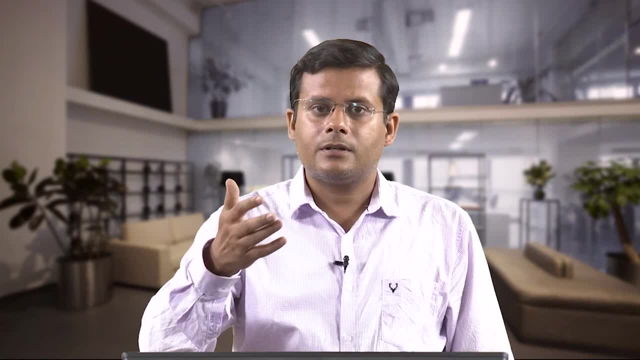 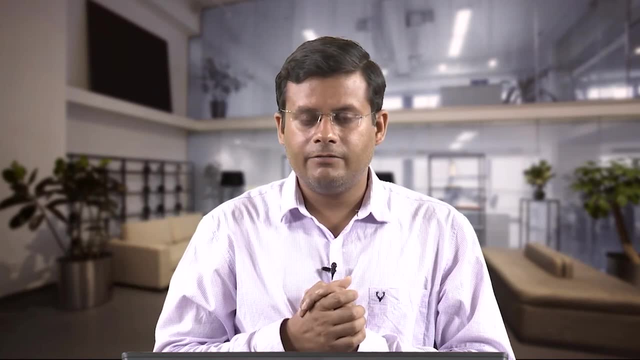 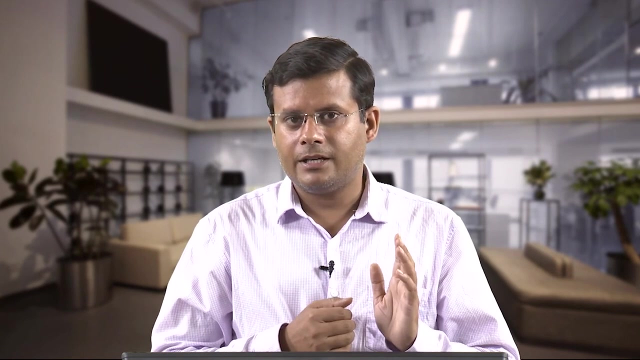 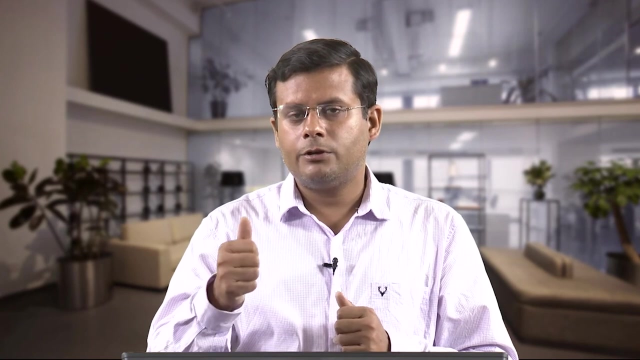 once you know the earlier orientation, then the wave would be polarized. Okay, I repeat it again, In an unpolarized wave, Okay, If you know the orientation of the electric field at some earlier time, then you cannot predict its orientation in later time. while in a polarized wave, if you know the orientation. 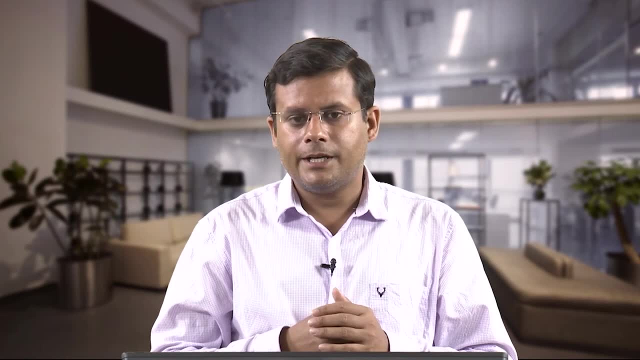 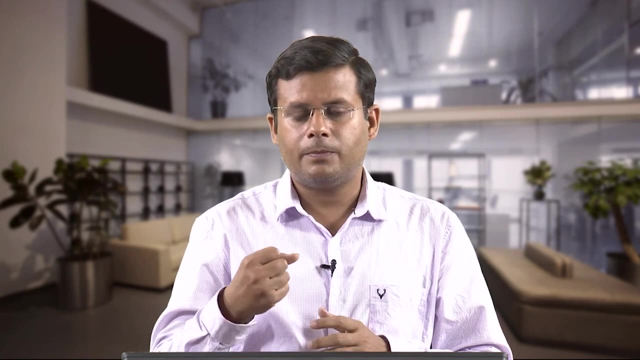 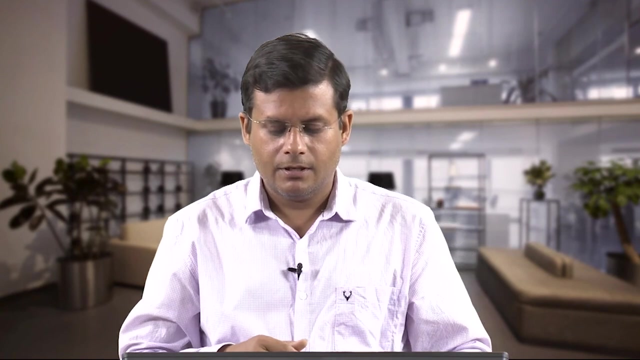 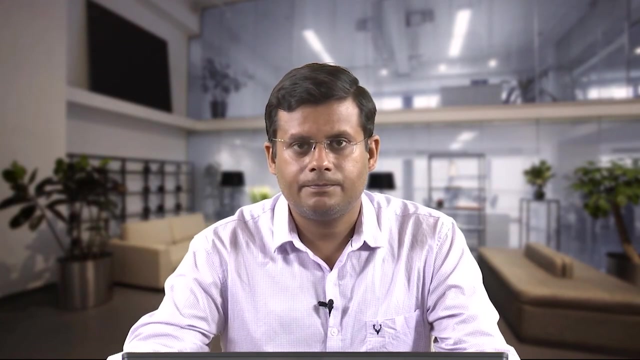 of electric field at some earlier point in time, then you can predict its orientation in some later point in time. This power of predictability comes in our hand once the wave is polarized. Okay, Having understood this, let us discuss the second type of polarization. 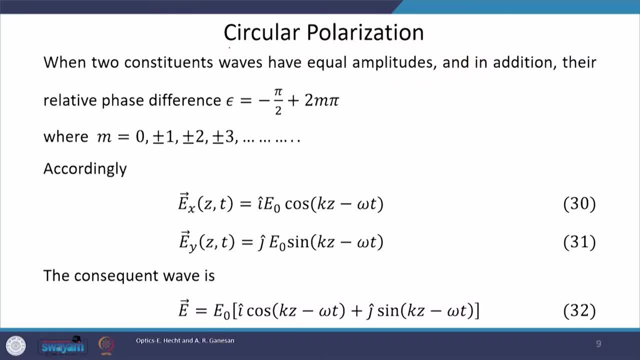 Okay, What is the second type of polarization? Circular polarization? Okay, Till now, we were considering two waves which were orthogonal, that is, they were oriented into directions which are 90 degree to each other. Okay, Okay, So they have two different amplitudes. 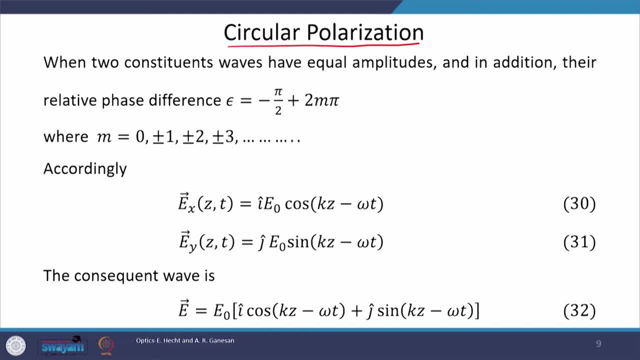 Okay, Now here we will consider waves which have equal amplitudes. E naught x would be equal to E naught y now, And we will assume that E naught x is equal to E naught y and it is equal to E naught. 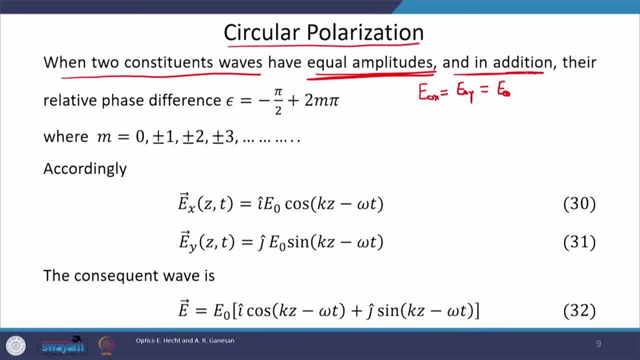 Okay, Okay, Okay. And in addition to this, their relative phase is equal to E naught y. Okay, phase difference, which is epsilon, is equal to minus pi by 2 plus integral multiple of 2 pi. Now let us consider the simplest case where m is equal to 0. then in that case the 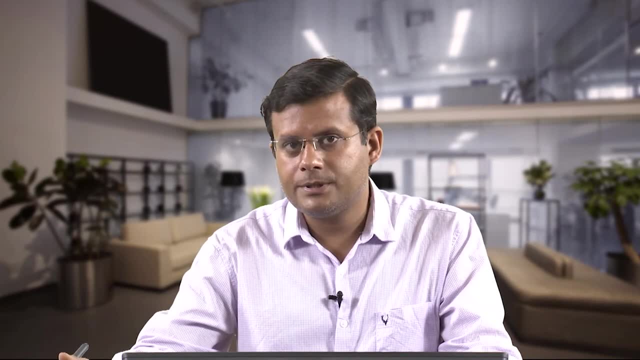 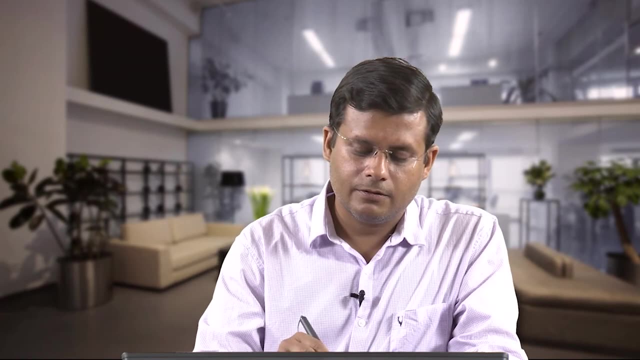 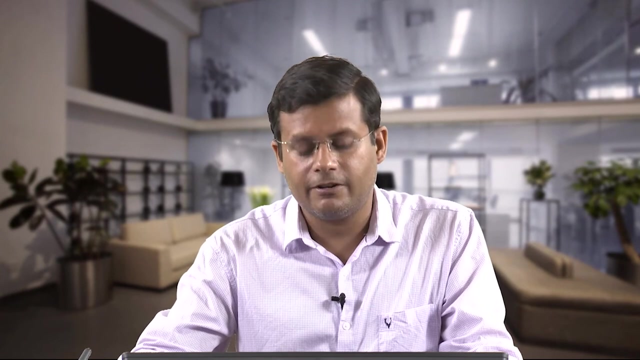 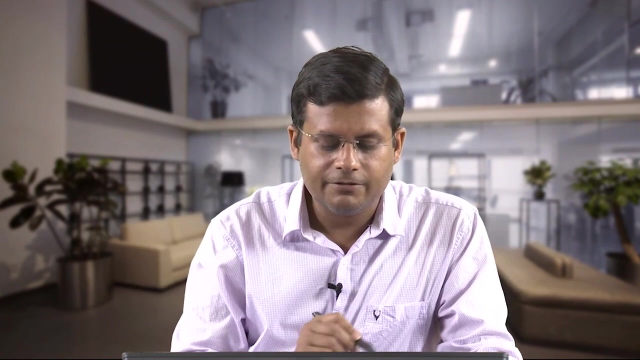 relative phase difference between the 2 orthogonal waves. the 2 overlapping orthogonal waves is minus pi by 2.. The simplest case is: epsilon is equal to minus pi by 2. with this let us rewrite the expression for wave. Two assumptions here are equal amplitudes and relative phase difference is minus pi. 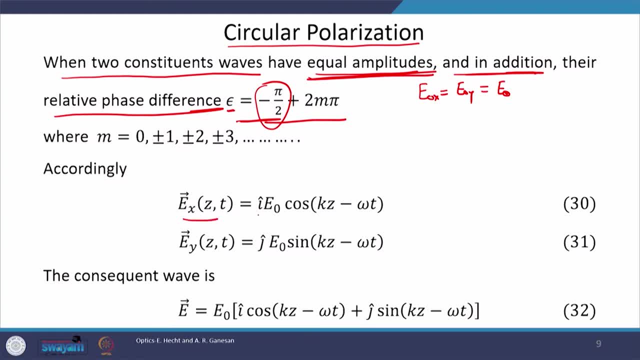 by 2.. With this, E x can be expressed as I into: E not, E not is here, and cos K Z minus omega t and E y is equal to J cap E, E naught again, and then sin kz minus omega t. no epsilon right now. Where is epsilon? 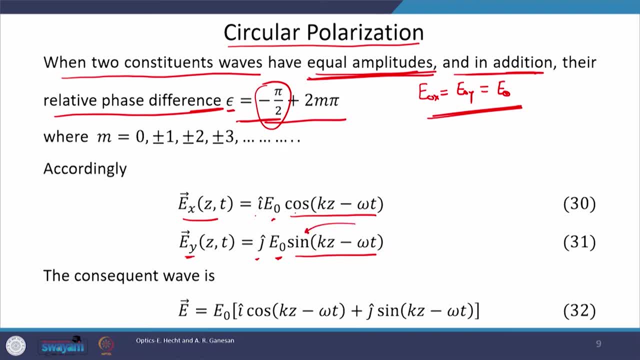 It is eaten up by this function. You see, in the first expression there is cosine term, while in the later second expression it is a sine term. Pi by 2 is now absorbed here in sine function and the amplitudes are the same as per our assumption. 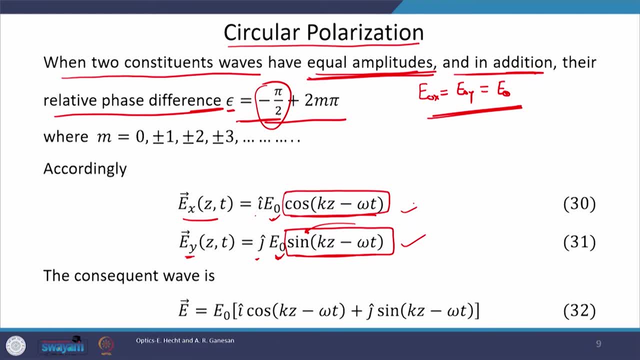 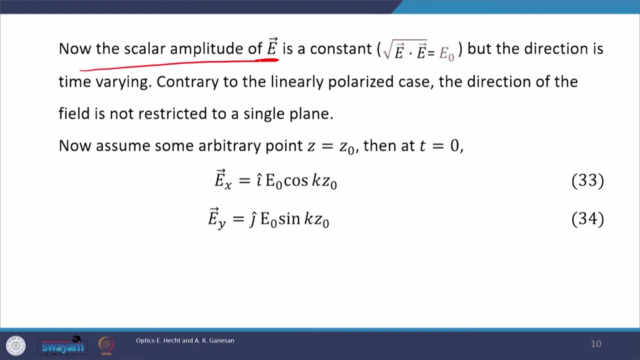 Now let us calculate the expression for the resultant disturbance. How to calculate? Add them vectorially. If we add them we will get this expression, the resultant one. Now it has e naught came out of the bracket. Why it is common Now the scalar amplitude of e. how to calculate the amplitude of e? 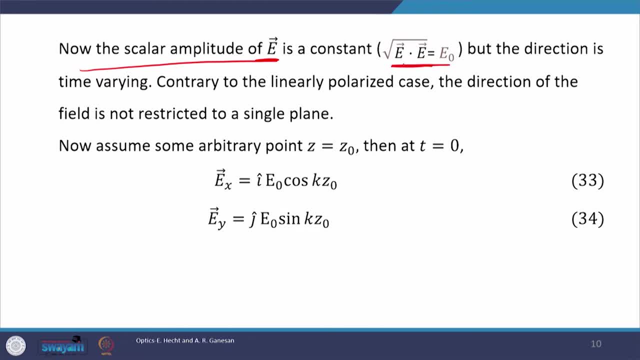 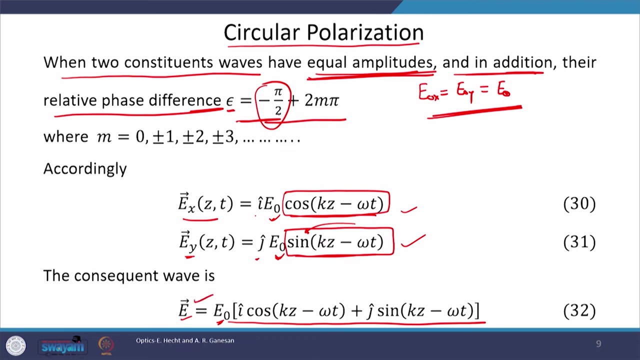 Amplitude of e is calculated using this formula: e is a vector quantity. Take dot product with itself and then square root it. This will give you the scalar amplitude of vector e. It is a constant. This resultant Okay. Vector e has an amplitude which is a constant, But the direction is time varying The direction. 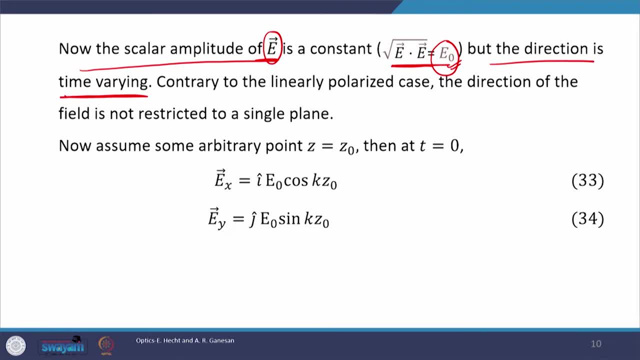 of e is now time varying. Now, contrary to the linear polarization case, the direction of the field is not restricted to a single plane. here I repeat for clearer understanding: The resultant field, e, you see, has a constant amplitude. The amplitude is not varying with. 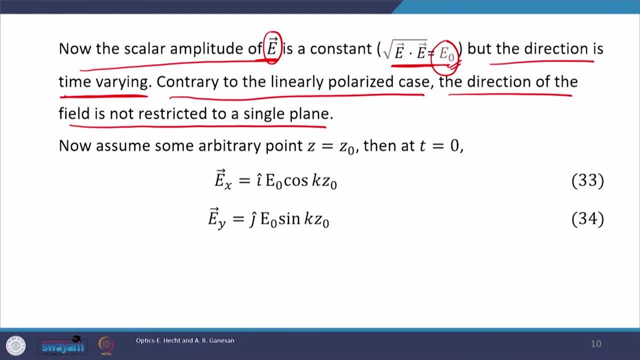 propagation or with time, But the direction of e field is now varying. Till now we were in the habit of seeing this kind of wave, whose amplitude is function of time. You see, the magnitude of these arrows are reducing here and then they are changing directions and 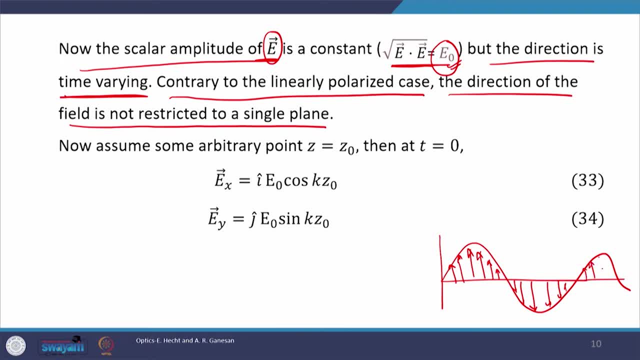 this is how we trace a sinusoidal wave, Is it? The amplitude was function of time? Whenever we say a field is a function of time, then it is amplitude which was varying with time or varying with z propagation space. But here, in case of circularly polarized light, what we saw is that the amplitude was Vereinhuis. 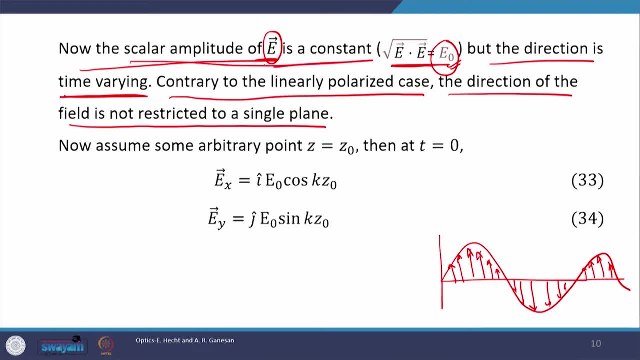 ++. Is it No? Yes, it is 2.. Is it Yes? S, 2. S, 2. S 3. amplitude is constant. it is not varying. Where does the time dependence comes in? The time dependence comes in from the time dependent direction In linearly polarized light: the. 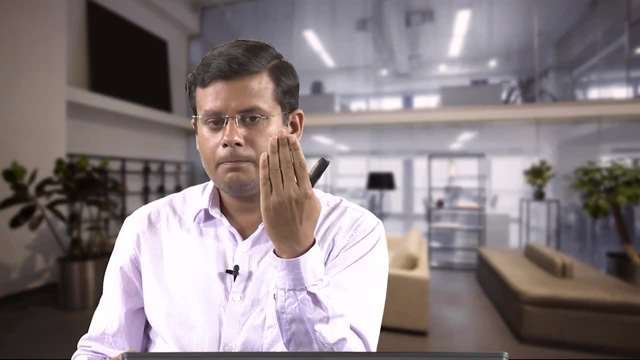 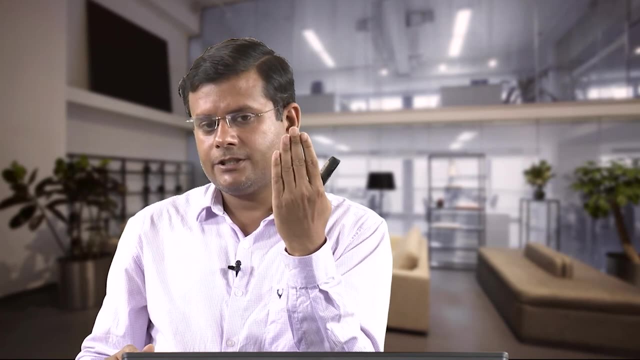 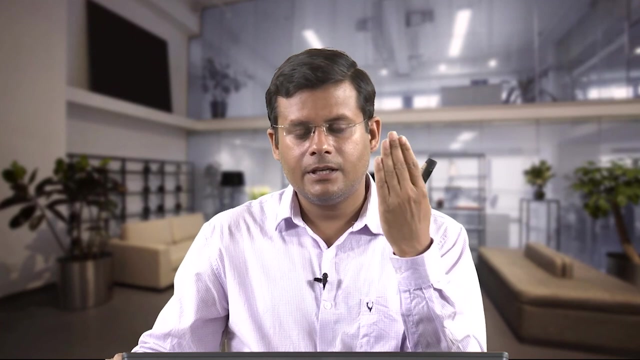 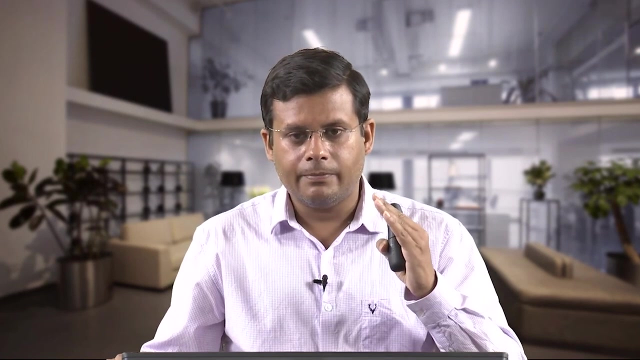 electric field was vibrating in a particular plane, its direction of vibration was not changing with the propagation. it was neither function of time nor function of space. But in case of circularly polarized light, the direction of E field is now changing with propagation. it is a function of time and space, However, its magnitude neither depends. 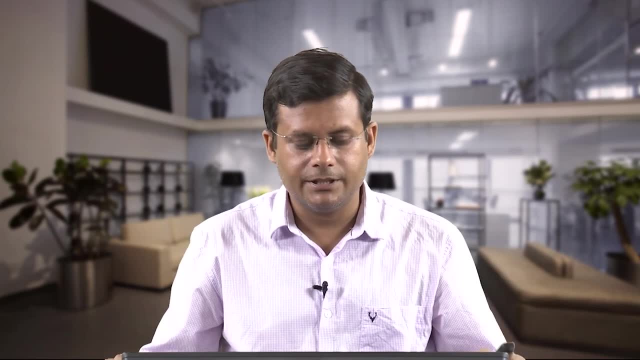 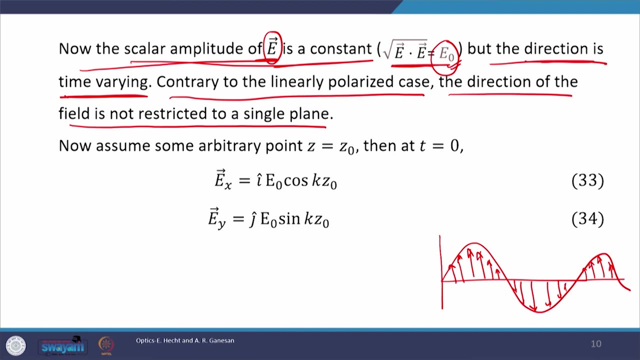 on space, nor in on time. it is a constant quantity. Now, with this in mind, Let us now assume some arbitrary point in a space, in direction of propagation, and that point is Z is equal to Z. naught, We are assuming that wave is propagating in Z direction and 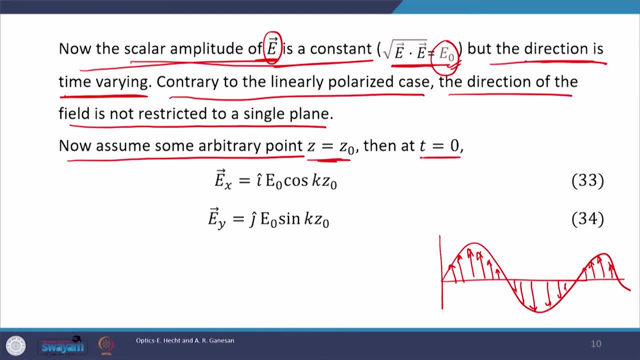 at a particular point, Z is equal to Z naught and at this point, when the wave reaches at point, Z is equal to Z naught. assume that the time counting starts from there, that is, time is equal to 0 there at z naught. 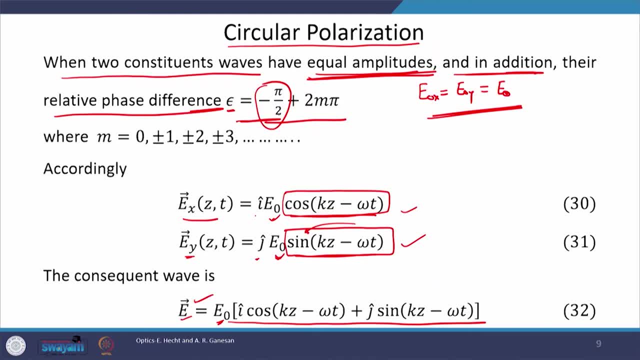 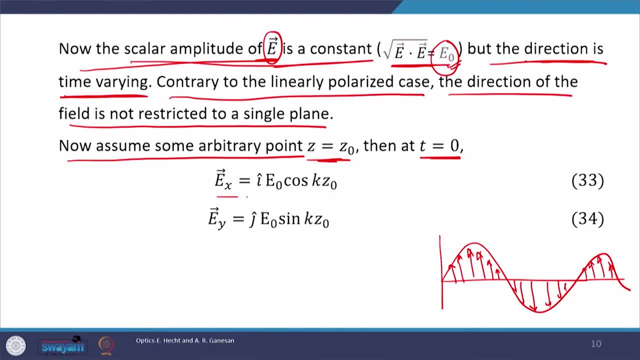 ________________________. ci is equal to z naught. Under these two conditions we can rewrite equation number 30 and 31, and new expression for e x. vector e x and vector e y are given by equation number 33 and 34.. 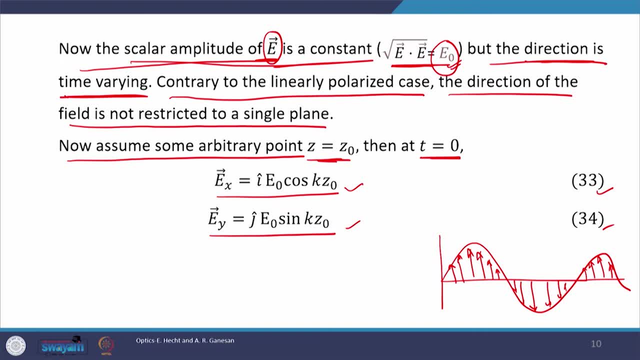 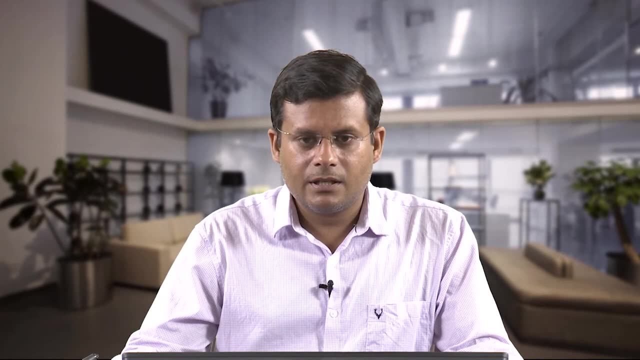 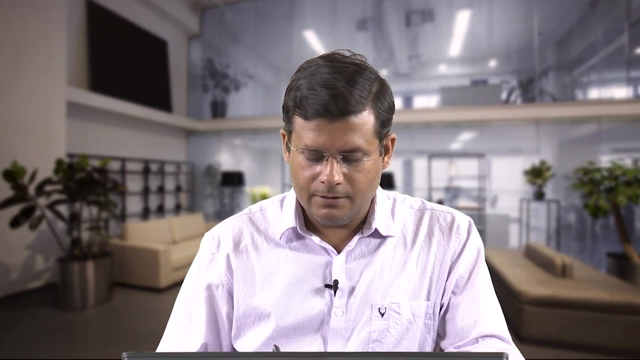 These are the two waves which will overlap. Now, if you square 33 and 34 and add them up, then you see that they traces a circle. It means the resultant would be a circularly polarized light, Because when you trace a circle out of the tip of the electric field, 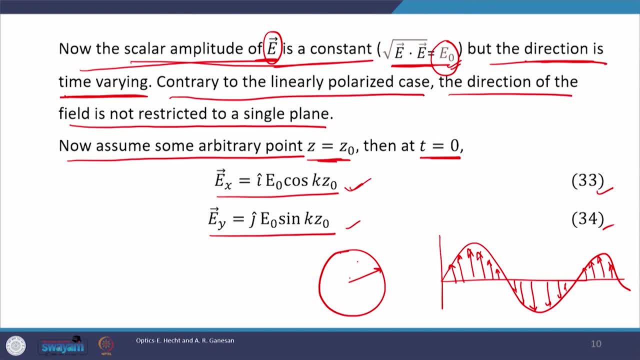 vector, Then the radius of the circle. irrespective of where you are on the circumference, the radius is constant. It is, it does not vary, and this is what is being said here also. The scalar amplitude is constant. Now, what is varying? The electric field vector will. 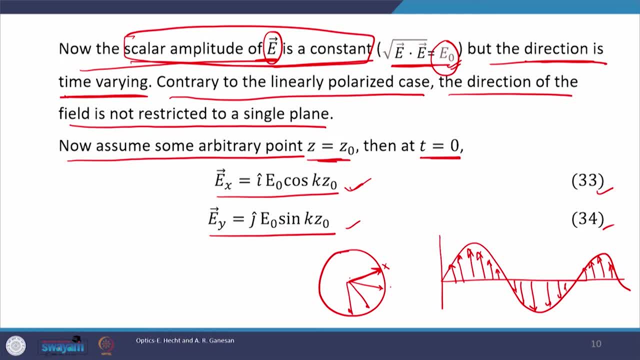 keep changing its direction. At some point of time it would be here, next here, next here. So it would keep changing its direction, But this change in direction would not be random. Why? If this would be random, then we would lose the power of predictability. 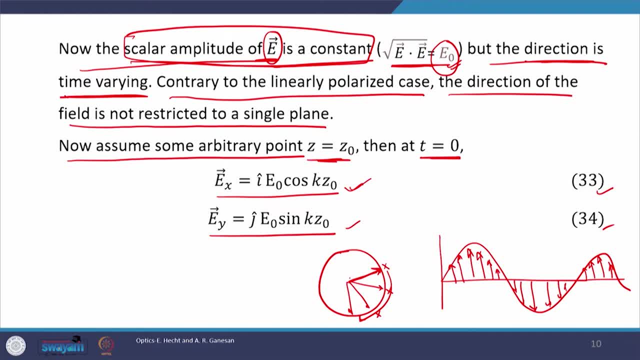 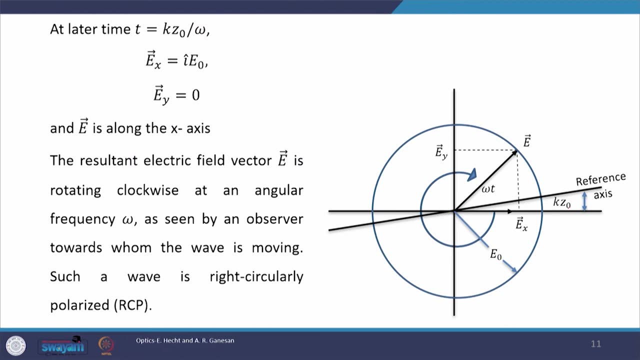 And we have already discussed that. if orientation of E field is predictable, then only we can say that the wave is polarized. That much information must be in our hand. Then let us see. let us see further, what happens with equation number 33 and 34.. 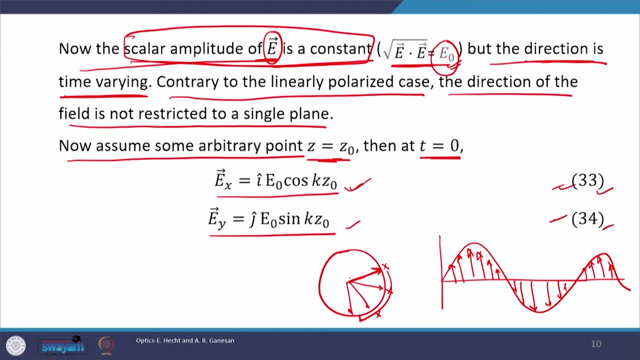 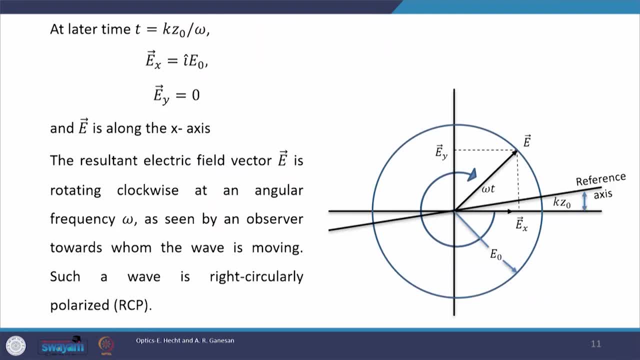 Equation number 33 and 34 is written at: z is equal to z0 and time t is equal to t0.. Now this particular point is given by this reference. Say, this is the reference on this horizontal axis. we expressed vector E on this vertical axis. it is vector E, y on horizontal. 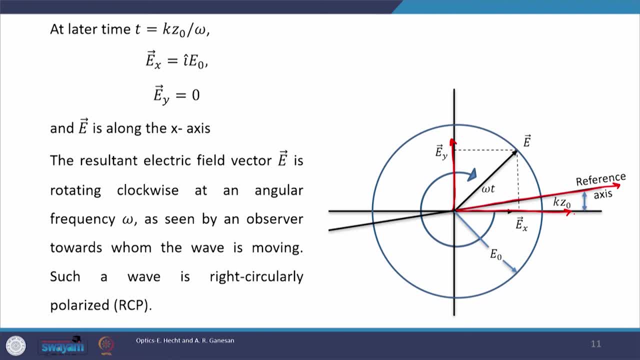 axis, it is vector E- x. on vertical axis, it is vector E- y and at certain point in space, which is z is equal to z, 0 and time t is equal to 0. Suppose this is the direction of the resultant field, which we call reference axis. Now, since this is the reference axis, we will 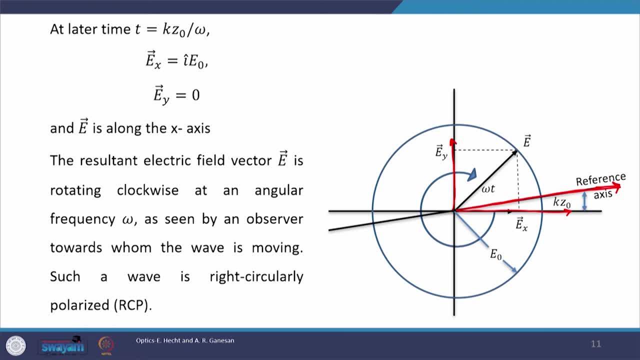 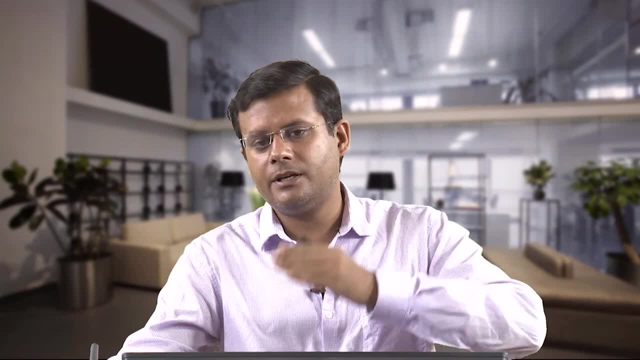 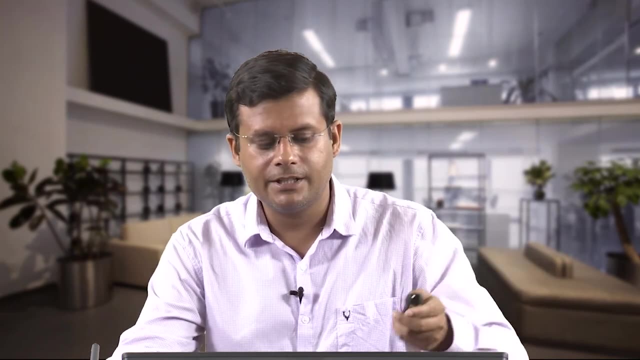 start the calculation from this reference axis, Since we are assuming time is equal to 0 here at this reference axis. as soon as we start from here, time will increase in positive direction here Now, time slowly will increase Now, suppose, at a lateral axis. 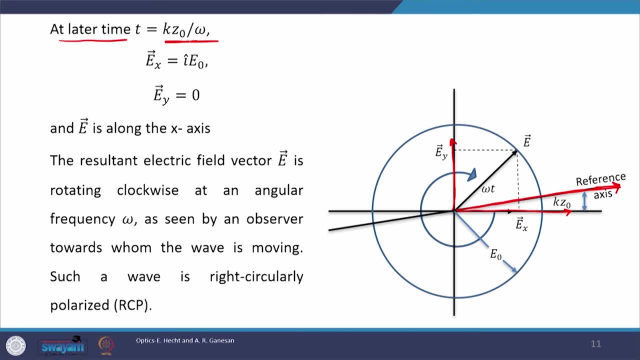 Suppose at a time which is given by k z 0, by omega. Where did we get this expression for from? we know that E is equal to E 0.. Suppose a vector quantity is here and then cos of omega t minus k z 0. Now how did we choose later time from this expression? When will 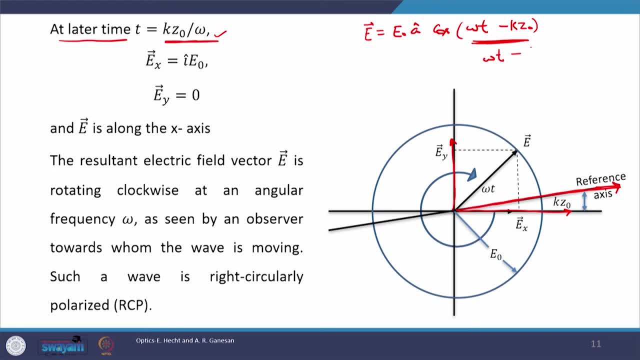 this expression will become 0?. This expression will become zero at a time point which is given by k, z, 0, by omega. okay, This we choose as our letter time. This is given here. okay, At this point, what will happen? The field? what will happen? The E x component? what is the expression of E x component? It? 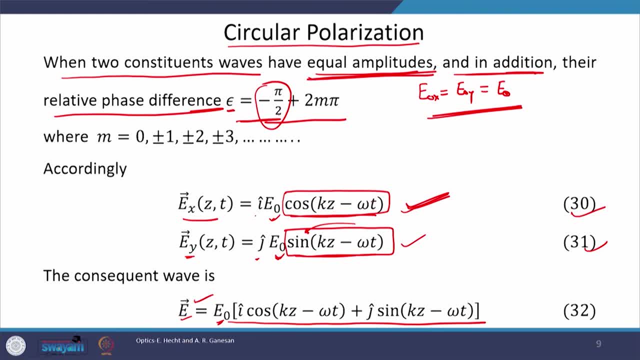 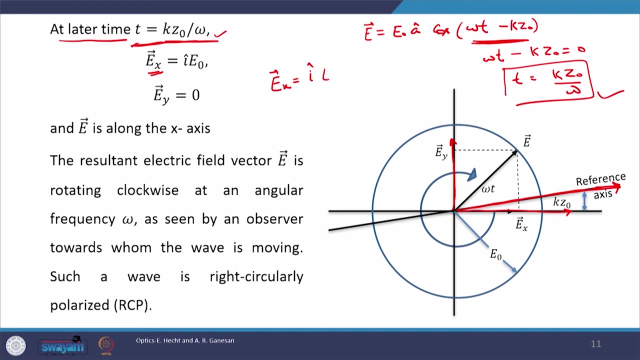 is given by equation number 13.. if you replace T by K, Z, naught, by omega here, then you will get 0 here. Now let me write it here for more clarity: E, x is equal to i cap, E naught cos, K, Z naught minus omega T. 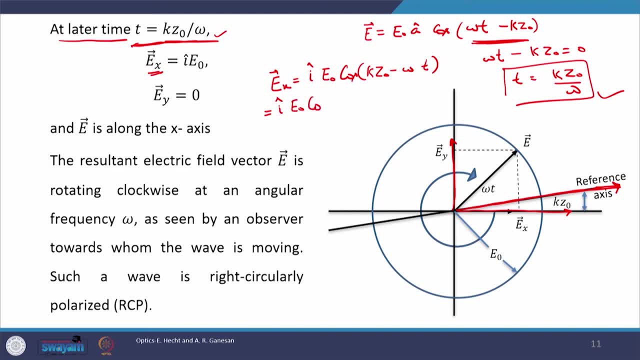 this is equal to: i cap E naught cos K Z naught minus omega. Now T has this value: K Z naught by omega. The omega omega will go away and K Z naught will go away with K Z naught. Therefore, we would be left with this value, and this is what is written here. Similarly, 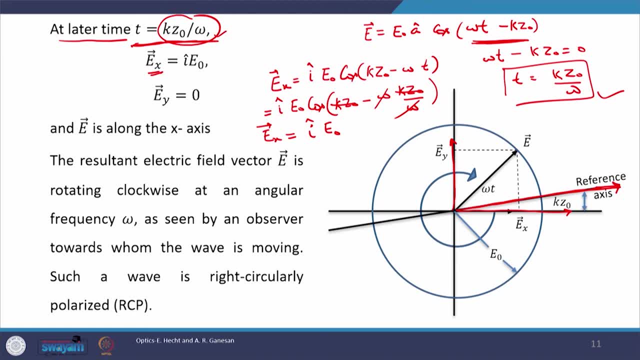 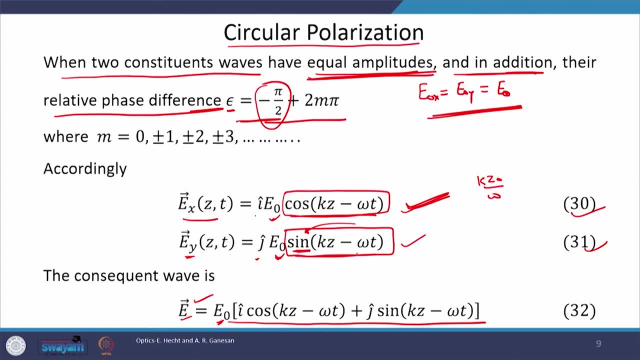 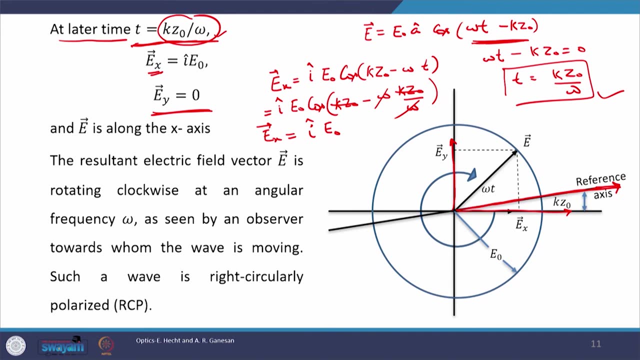 we can calculate E y. If the phase is 0, then sin which is sitting here, the sin of 0, would be equal to 0 and therefore E x- sorry. therefore E y would be equal to 0. And therefore at: 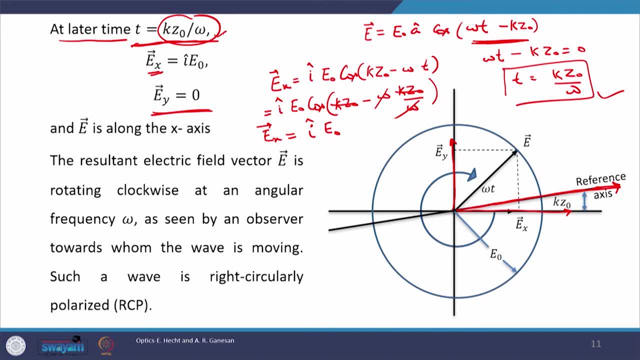 a later, initially Order of magnitude 2,. the wave was initially along the reference axis direction and at a later time the x component has some finite positive value and the y component has 0 value. x component has some finite value and y component has 0 value. It means from the reference. 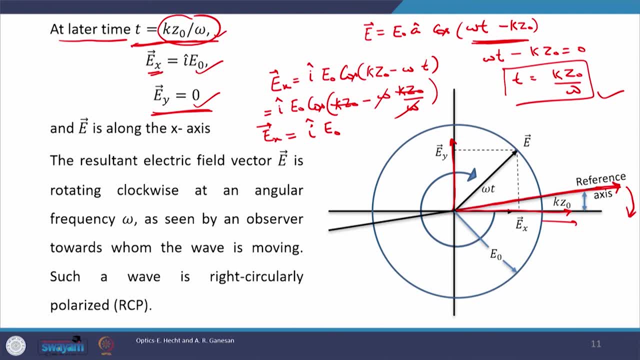 axis direction. wave, rotated wave came here in this: the electric field, the electric field resultant electric field rotated in this direction. E x per k z naught by omega T is equal to i cap A naught minus omega T, And therefore 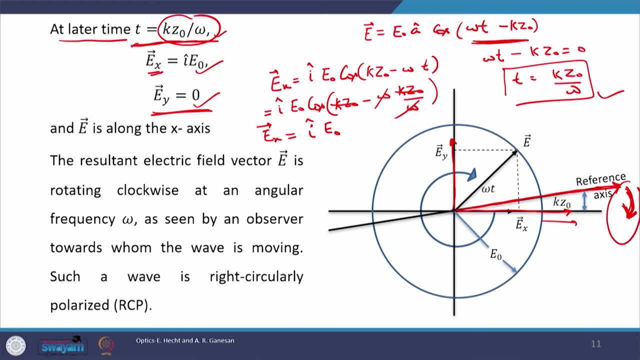 rotated in this direction, as shown by this arrow here. Initially it was in along reference as axis direction. Now the resultant is along E x vector direction and therefore the resultant is along the x axis. Therefore we can say that the resultant electric field vector E. 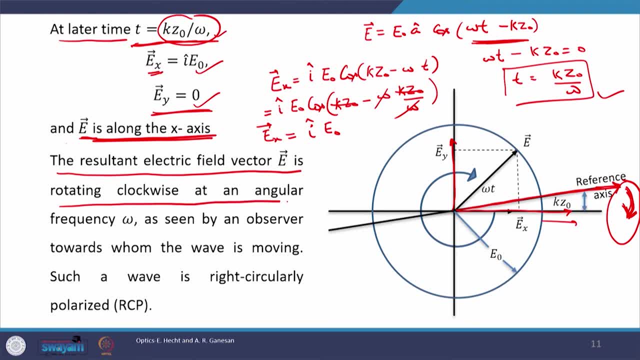 is rotating clockwise direction at an angular frequency, omega, as seen by an observer towards whom the wave is moving- a very important concept. Initially, the wave was along this reference axis direction. Now the wave is on x axis and the resultant E is pointing. 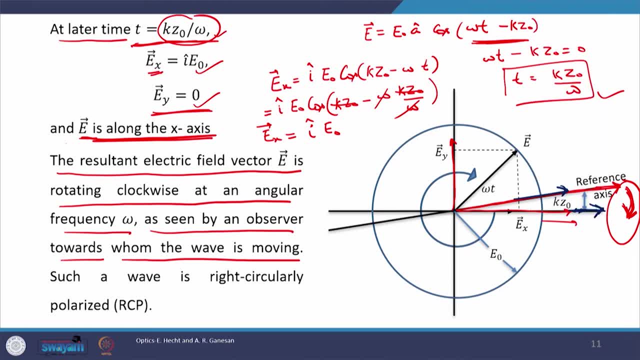 along x, E x vector direction. The whole rotation is clockwise fashion. This is how the wave is rotating. The rotation is like this, which is clockwise rotation, and we are standing in the front and we are looking into the source. The light is coming towards us and, as an observer, we are looking into. 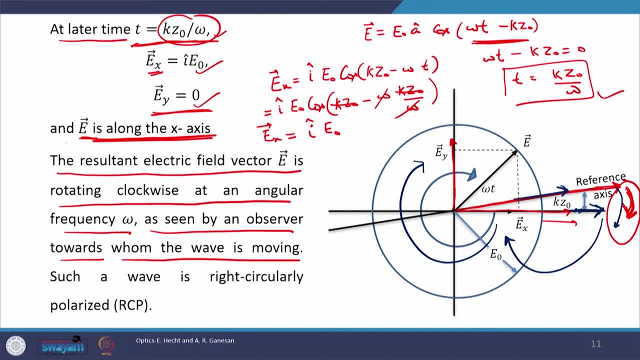 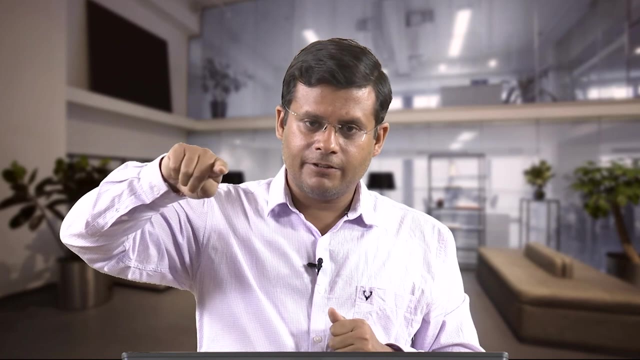 the source. Under this case, if we see the resultant electric field, vector E, x vector is rotating clockwise direction, then such a wave is called right circularly polarized wave. I repeat, if we are looking into the source and seeing the resultant electric field, 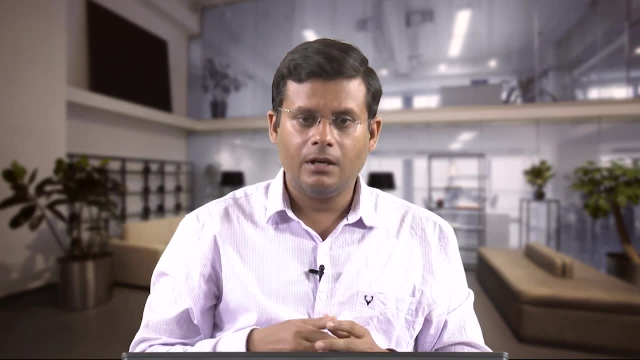 is rotating clockwise direction or, more accurately, the tip of resultant electric field vector is rotating clockwise direction, then such a wave is called right circularly polarized wave. I repeat, if we are looking into the source and seeing the resultant electric field is rotating clockwise direction or, more accurately, the tip of resultant electric field vector is: 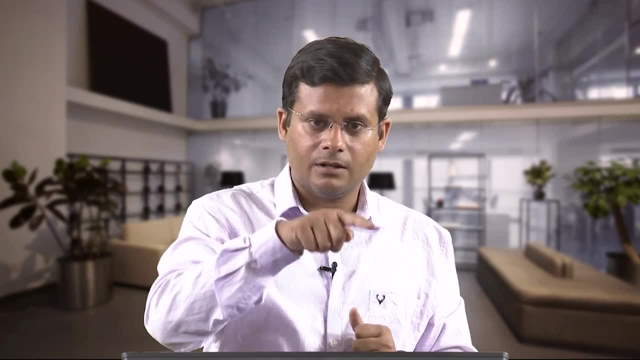 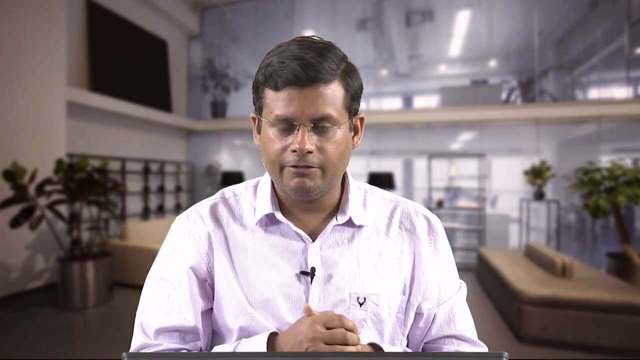 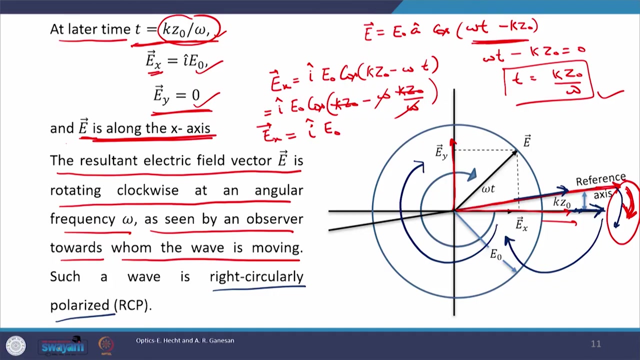 field vector is tracing a circle in a clockwise direction, then this kind of polarization or this kind of wave is called right circularly polarized wave, And this is also very much clear in this figure. The tip of the electric field vector is rotating in a clockwise fashion. In the case when we are looking into the source, the light is 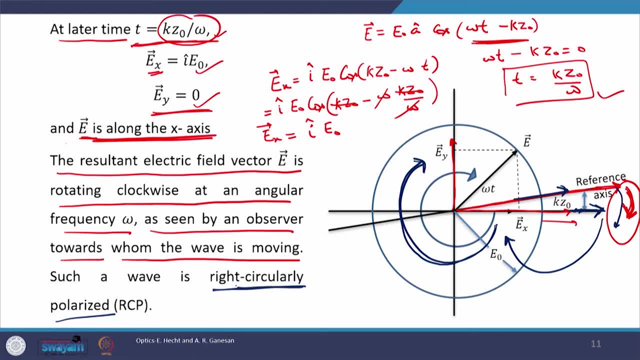 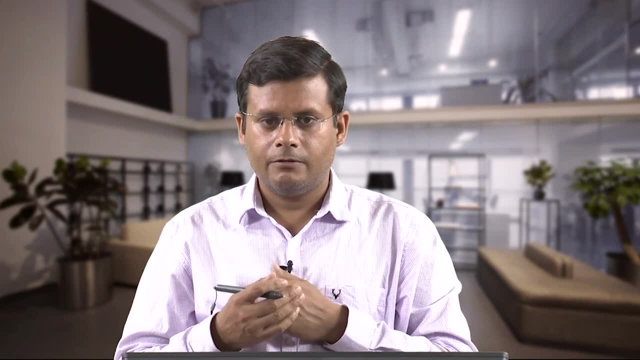 coming towards us and this wave is called right, circularly polarized. This is a very important concept. We must look into the source and light must be coming towards us. Therefore, the referencing is very important. We must look into the source, Light must be coming. 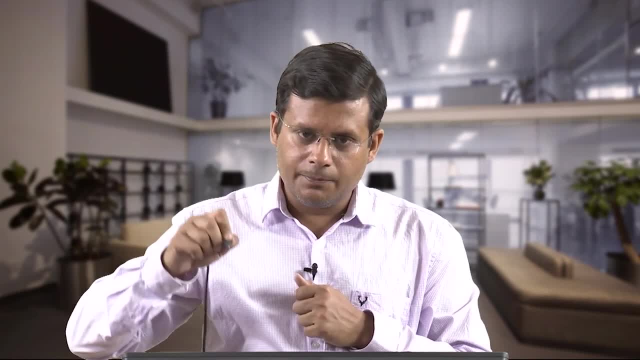 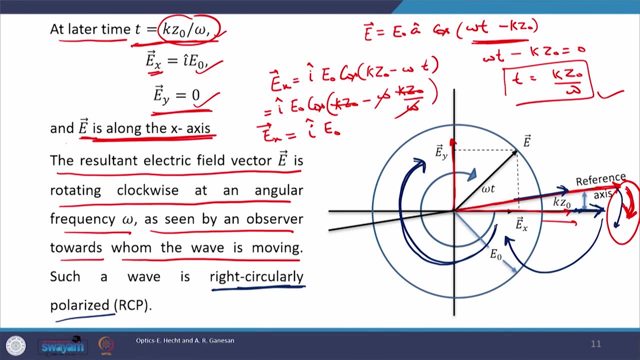 towards us and under this condition, if the tip is rotating in a clockwise fashion, then the wave is called right circularly polarized Right circularly, then the wave is right circularly polarized wave. The acronyms for right circularly polarized wave is RCP: right circularly polarized. Similarly, if the relative 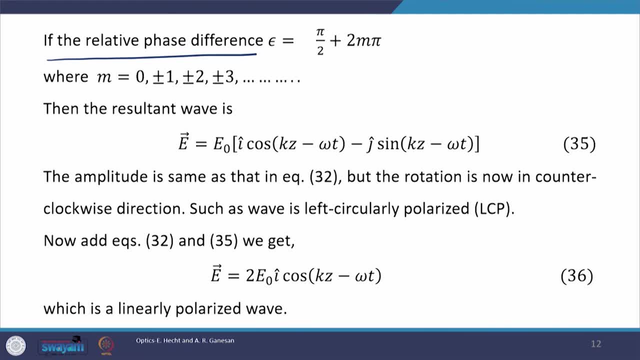 phase difference is pi by 2 and then integral multiple of pi, then what will happen is that there would be a minus sign here instead of plus sign. The resultant will have minus sign, And if this is the case, then the resultant will trace the tip of the resultant field. 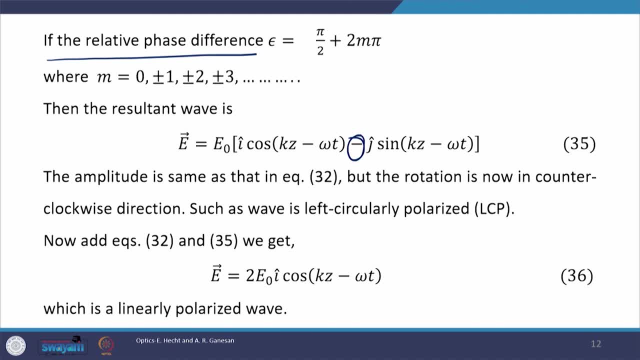 will trace a circle in a anti-clockwise fashion, And such a wave is called left circularly polarized, or LCP. Earlier it was RCP, Now it is LCP. Now- this is equation number 35- represent an LCP. 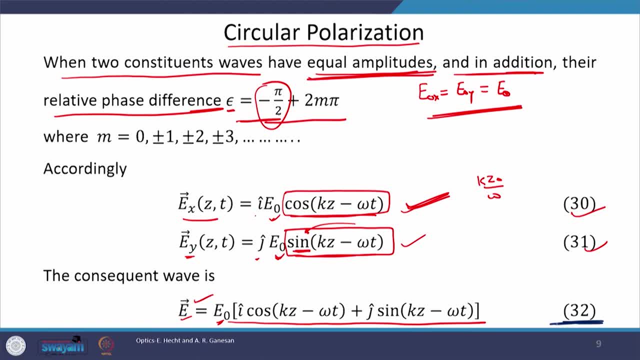 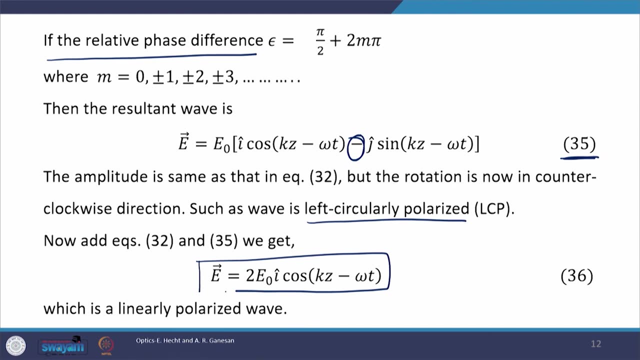 Now let us add these two equations here. The only difference here is in sign. Now, if we add them up, this is the resultant. If you add LCP and RCP, then you get equation number 36, which clearly is pointing along X axis and which is a linearly polarized 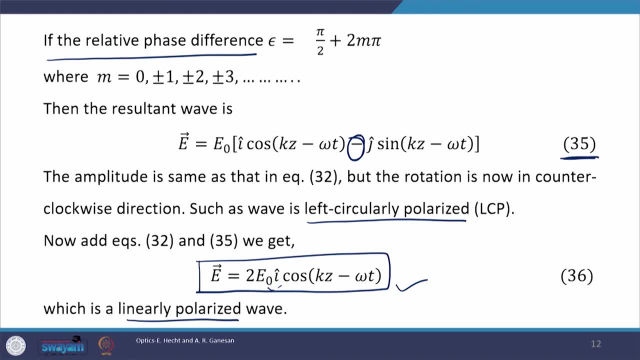 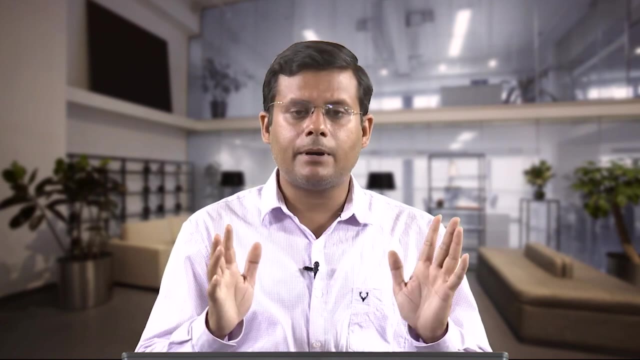 light. Okay, Which means out of left circularly and right circularly polarized light, we can again generate a linearly polarized light. A more generalized statement is: using two orthogonally polarized light, we can generate any type of polarization or, alternatively, any type of polarization. 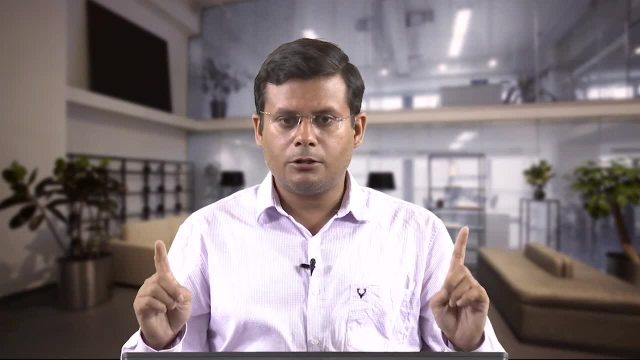 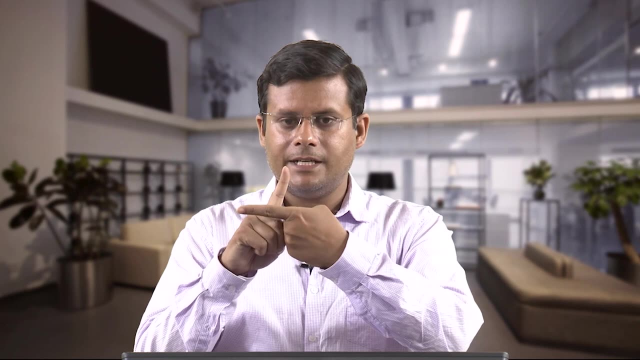 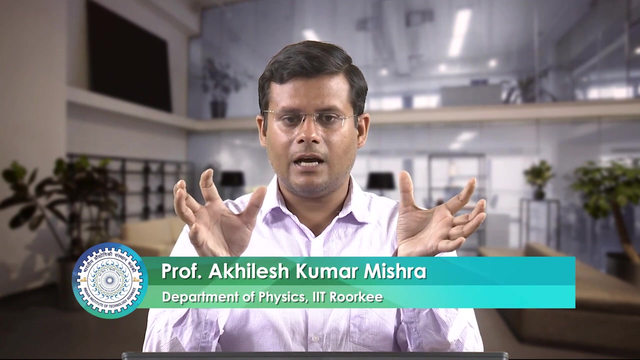 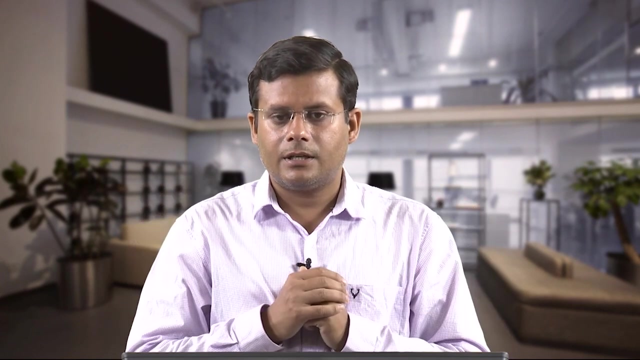 can be expressed in the form of orthogonally polarized light. Okay, X polarized and Y polarized light are orthogonal. Left circularly polarized and right circularly polarized light are orthogonal. So using these two pairs we can generate any kind. 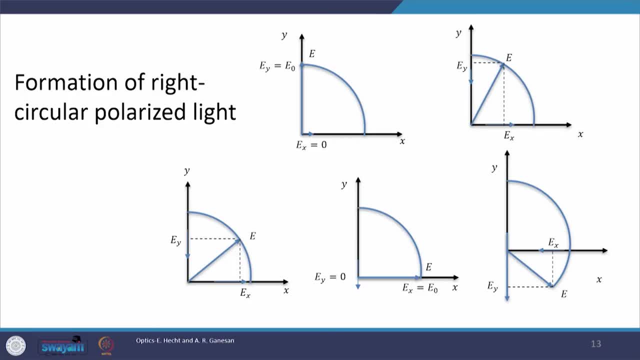 of polarization. Now you can see here the formation of circle in a circularly polarized light. You see at some instant where, suppose, t is equal to 0. Okay, Okay, Now you see that Ex is equal to 0 and Ey has some finite value equal to E0.. Therefore, 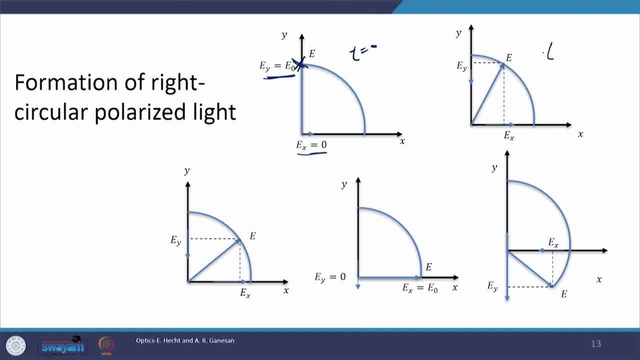 the resultant would be here At some later time. suppose t is equal to delta, t Ex has gained some value and E0 is reducing. Therefore the resultant is not now pointing towards Y axis. It has this orientation now. It has rotated clockwise fashion. Now again, if 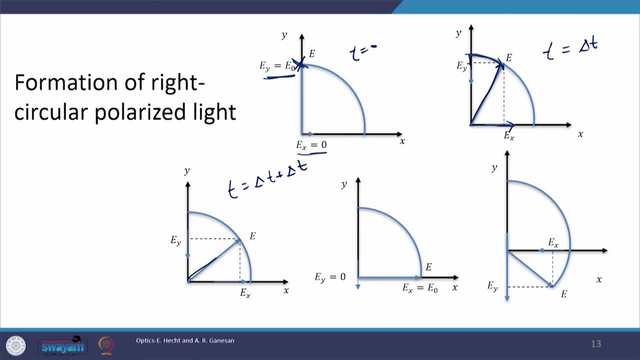 you move further, delta t will be here, Okay, Okay, So delta t plus delta t. resultant E came here. Now Ey is reducing down and the resultant in slow is, in the next interval of time, delta t plus delta t plus delta t, suppose. Now. 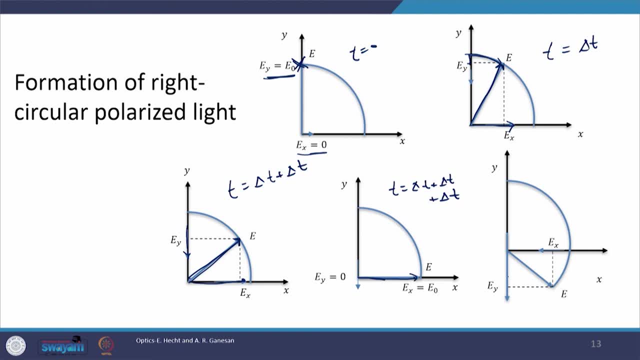 E is now is along X axis and slowly you are seeing that it is tracing a circle, with propagation, Okay, And this particular light is doing clockwise, Okay, Okay, Okay. So this is the rotation and therefore it is called right, circularly polarized light.